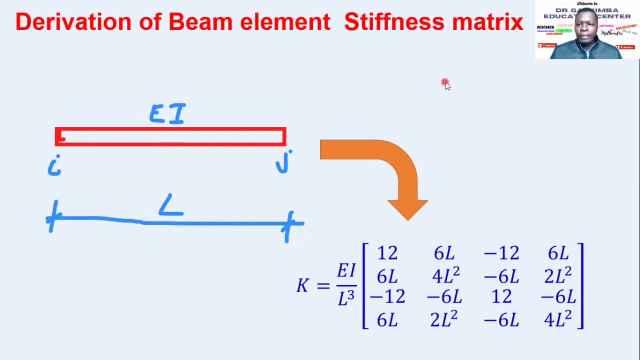 And before we start, let's remind ourselves. of course, in that lesson you're going to also refresh again, But let's remind ourselves of a few things here. Number one is that the notation. okay, let's consider the positive notation or the positive sign convention. 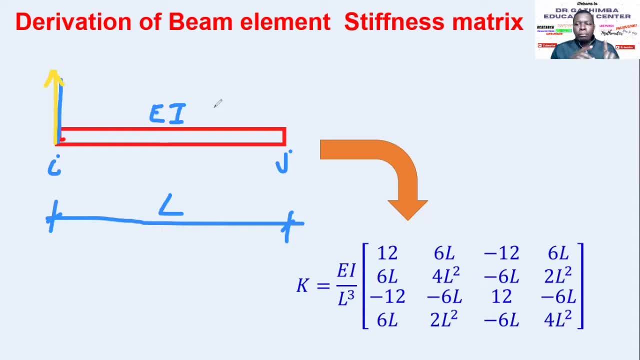 For the case of the, there was a case of the finite element beam analysis and also the one that we already covered in strength of materials, where you talk of the beam theory. So there was kind of a slight difference. So watch that video. 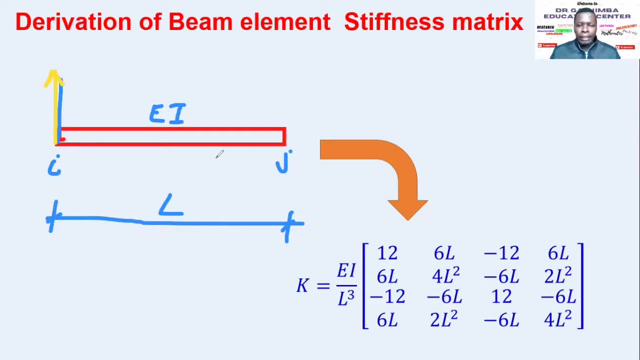 Also there are three. I will leave the link in the description box And, that being said, let's just highlight here that positive moments are counterclockwise, so they are moment like that and either node, Then positive forces, or shear forces, or active forces, I mean electrophoresis. it will be upward, okay. 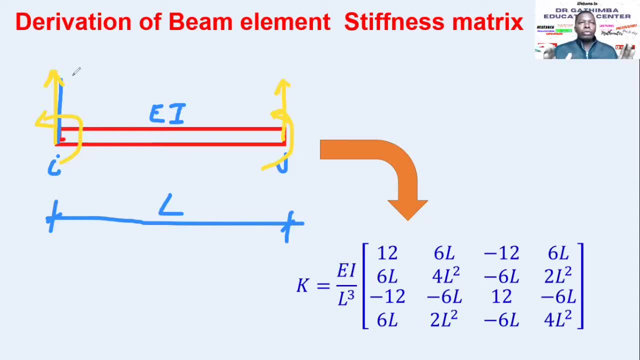 So this is for the finite element, But you know, for the Beam theory, we talk of hogging moments being a diff and sagging moment being positive, And of course we talk of the forces in the counterclockwise direction. 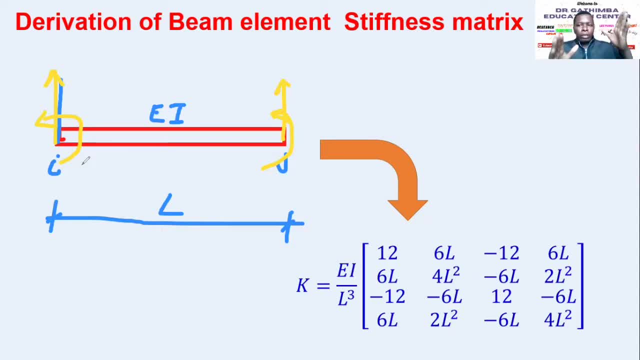 For the shear forces and the applied loads in the counterclockwise direction they'd be positive. But in this case, for the finite element- beam analysis- upward forces are positive. So for the beam element we talked of there are two degrees of freedom. 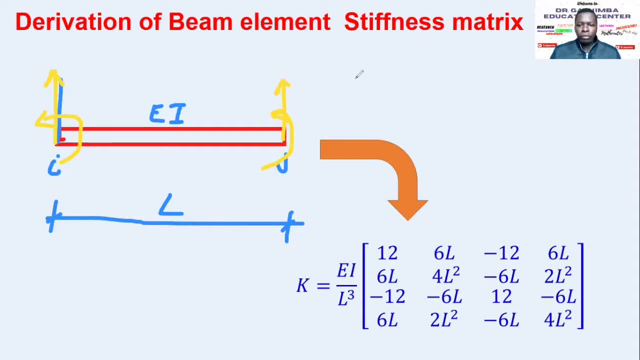 And each node and these degrees of freedom of course they are represented by, there will be displacement and rotation. So in either node we shall have displacement, small v up one. Remember now, in beam we are not in actual like the bi-elements, it's a transverse load. 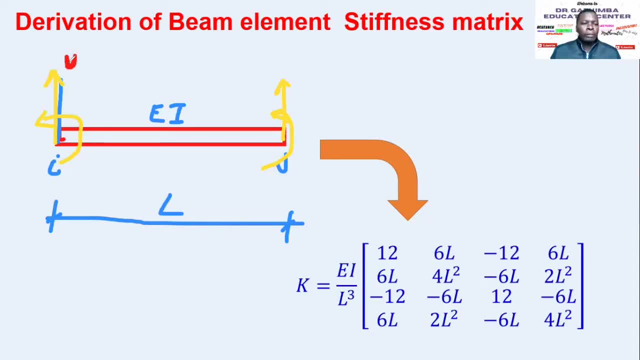 So there will be the rotation, there will be the actual, I mean the deflection v and the rotation theta due to the moment, And, of course, now the external quantities, Because remember, finite element, The equation, the equilibrium equation, f is k delta. 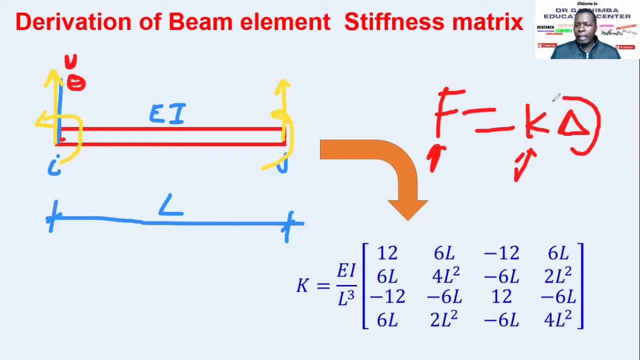 These are the external components, This is stiffness, And then these are the displacement component. So the displacement are transverse displacement and the rotation And the external vector for node of forces. these are the moments. You have the moment. So if you take this as the y direction, this direction as the x direction, 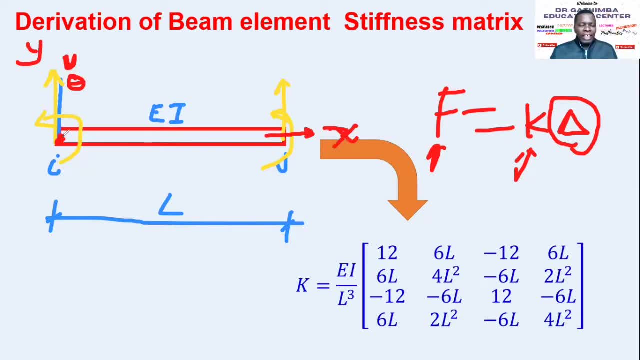 So towards the paper. if you consider Towards the paper, that's the z direction And therefore the moment are rotating about the z axis. okay, or the z axis, So we have the moment, positive moment, like that, even in this case, like that. 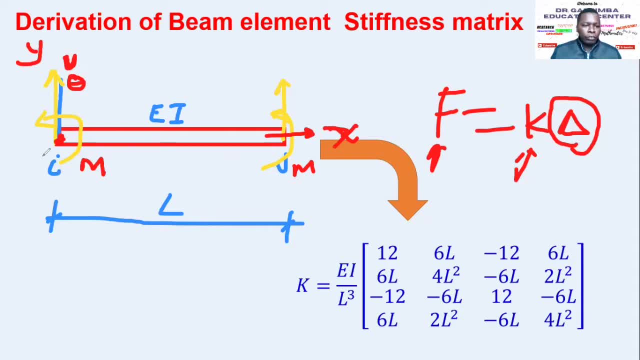 And then rotation: okay, the externally applied force. of course, if it's fixed head here, this will be the reaction moment here And on this side it depends with the support condition. We are just taking an element. we don't know which side is fixed, which is free. 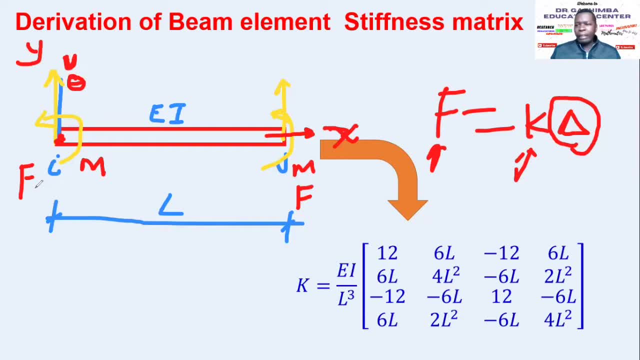 Or both of them are supported. So in that case we can either have f being the reaction or being an externally applied force, which can be equals to zero if there is no force applied there. So this is the beam element, just a refresher from lesson number three. 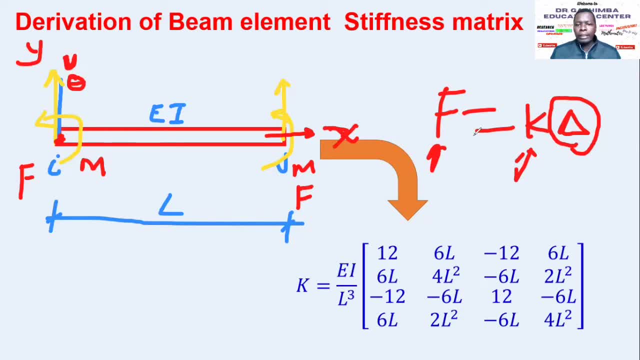 And lesson number four. sorry, is it four? Yeah, yeah, Actually it's not lesson number four, It should be lesson number, because in lesson number one was introduction, two was in the spring element, three was in a bar and four was bar in 2D. 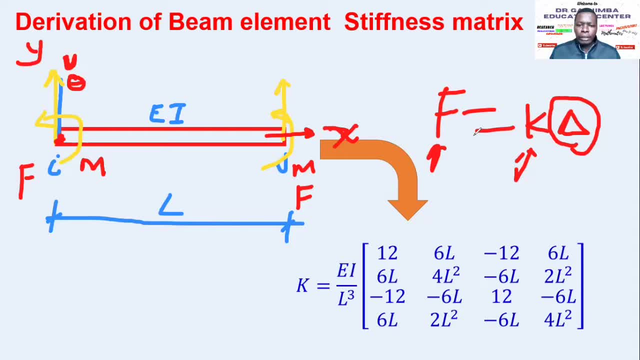 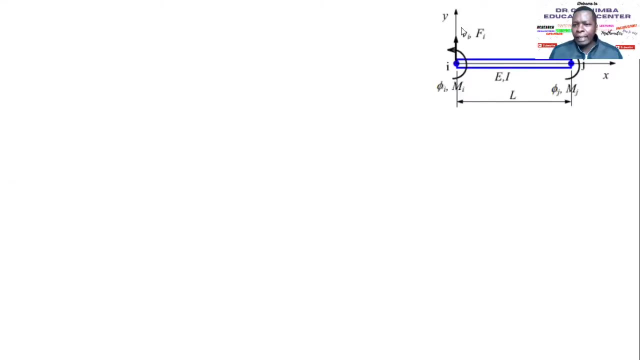 So it's lesson number four. let's say that, Okay, basically click the link there, All right, and with that let's dive in. So this is what I have just given as highlights. You have this At the nodes we have, and maybe I should now remove this, my video here, so that we can see that. 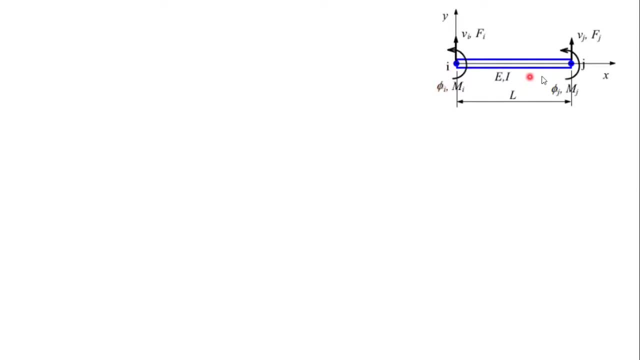 So we have, at each node, we have the external, Of course, the displacement component. this would be the rotation theta, and here we are using phi, can use phi or theta- and then the vertical component of the displacement: v for each node, i and j, so two degrees of freedom. 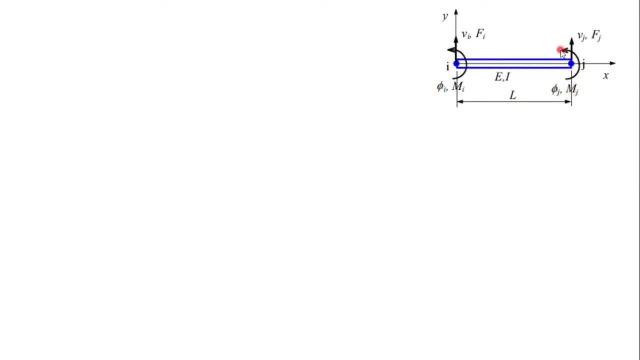 External nodal quantities is the moment. m are about the z-axis. You can see the y-axis upward, the x-axis is horizontal, so the z-axis is toward the plane of this paper, And then, of course, for moment, we'll bring about rotation. 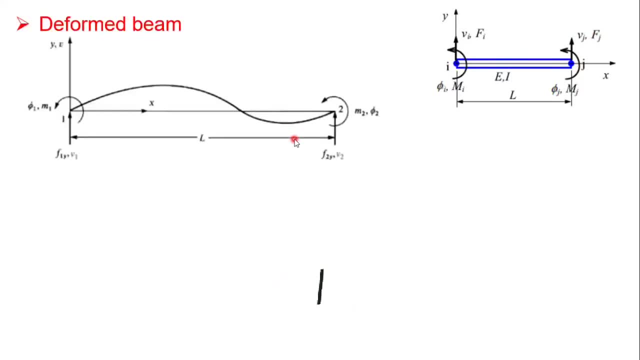 External forces, every bit of multi-displacement Now, because of these applied forces, this is what we could expect as the deformation or the deformed shape. The positive moment like this, the positive moment, would be about the positive rotation. Yeah, so, measured from the horizontal axis, counterclockwise, that is the positive rotation. 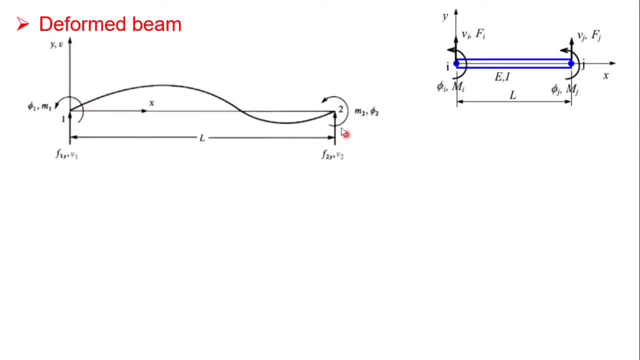 That's why we are saying now this would be a positive angle, theta phi one. and this here is positive phi one. That's why we are saying now this would be a positive angle, theta phi two. Shear forces, or axial, or load. I mean not axial, lateral load. 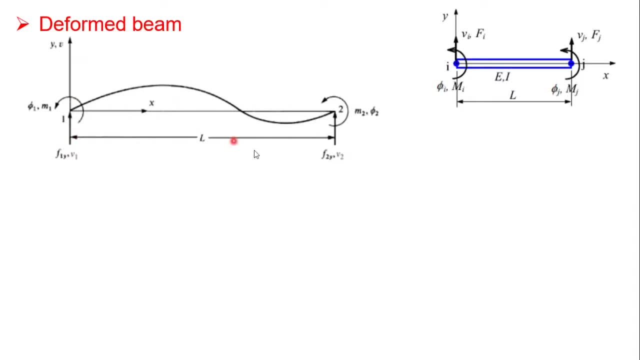 So in this node we have the f one and this one, f two, so acting upwards, that is positive. So because of these positive quantities that are applied, then this is a typical deformed shape that we anticipate. All right, so relate what is applied here. what is a deformed shape? 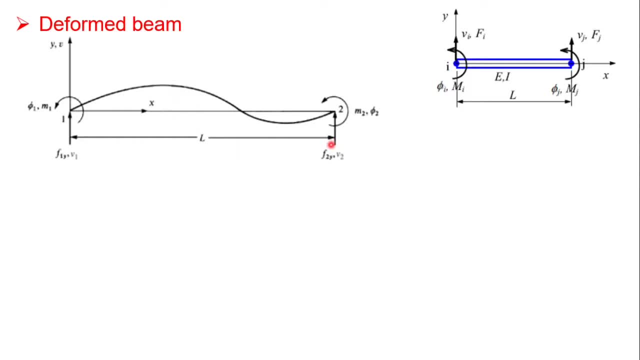 And, as you can look at this, it's curves twice, so up one, down one. This, if you remember your maths, well, this is the typical of a cubic expression. And so what does this tell us? So, if we remind ourselves, on lesson number, I believe it should be lesson number three or two. 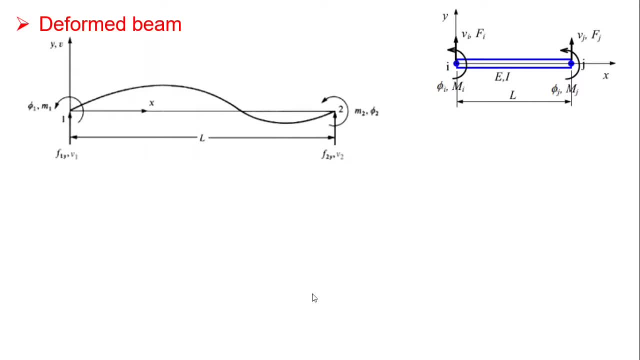 we talked over the. of course, we started from the first one. we talked about the displacement function- We need to set a displacement function, okay. And we talked over the displacement function in finite elements. We take a polynomial that tries to define or describe the interpolation between two nodes. 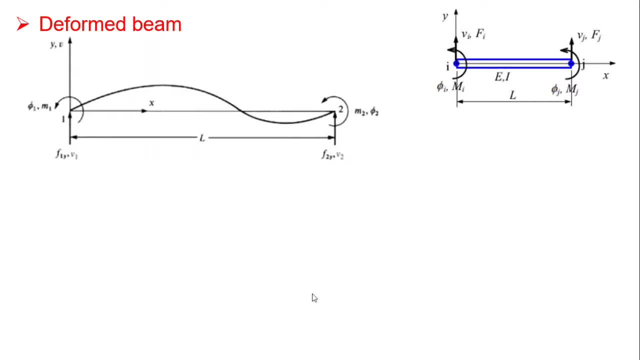 because we say the exact values or known values are only between nodes. So in between the nodes we need to interpolate And that we use a polynomial that describes the shape or the distribution of the displacement between the nodes. And in this case we talked of for the bar element it was fixed like this: 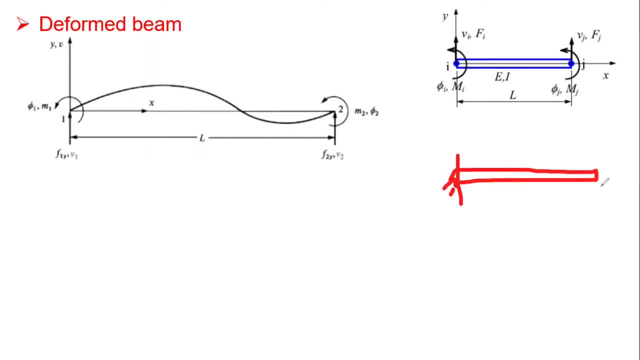 and then we added the linear function. okay, So we are saying this is 0, and we talked of a linear elastic. okay, So it will base the whole clue, So the irrigation continue like that, okay, So what did you say this? 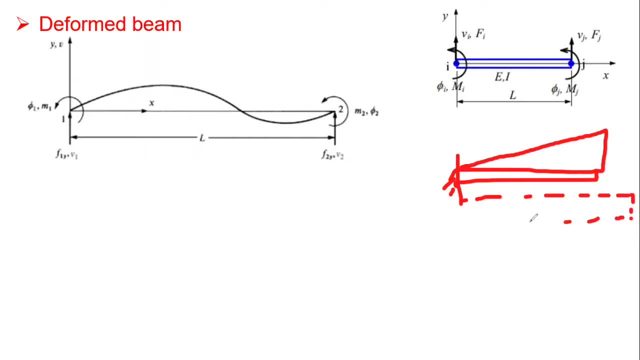 So the irrigation of the bar is like this. so you can consider the bar which is irrigated like this, But because we know the irrigation is linear, so we can say from this side is 0, and from this side is the maximum quantity we are getting here. 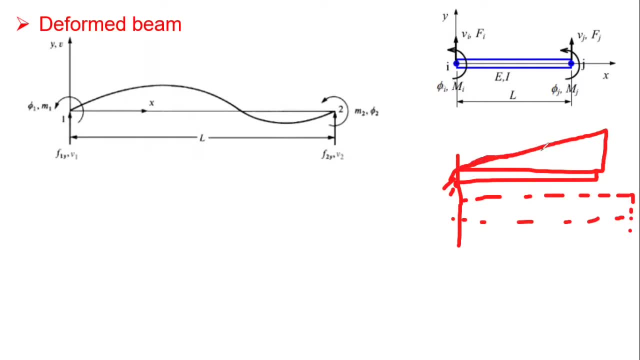 So it's varying linearly and that's why we're able to describe these displacement functions as a linear equation. remember, y is equals to mx plus c. so we we employed this, so we said maybe y is equals to a plus bx, like that, and we calculated the values of the coefficient a one and a two. 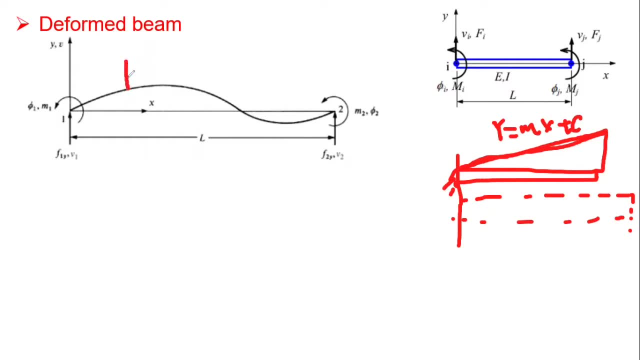 similarly for the beam element. if you look at this, if you look at this, this is a cubic expression, so it means our, we can assume suitably assume our displacement function to be of the form, a polynomial of order, three: a x squared plus b x, a x cube plus b x squared plus c x plus d, or in in. 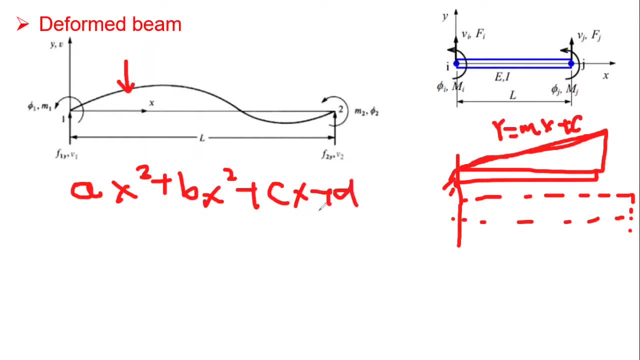 this case, you can say a1, a2, a3, a4. these are just coefficients. so we thought: now you know what you are. we are doing in this case. we just, you just need to. we follow the procedures that you follow for the environment. you just need to calculate what are these values of. we express the values. 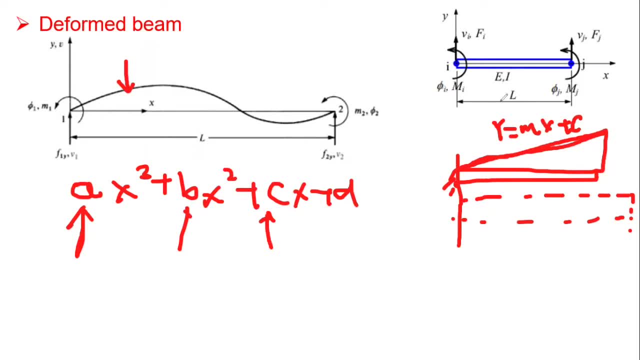 of the coefficient, in terms of what is given, what will be known, so, of course, in terms of the length, in terms of rigidity, in terms of uh, the nodal quantities, phi and uh and and v, small v there. okay, so that now we can express, we can read over the unknowns: a, b, c, d. we express them in terms of one node. 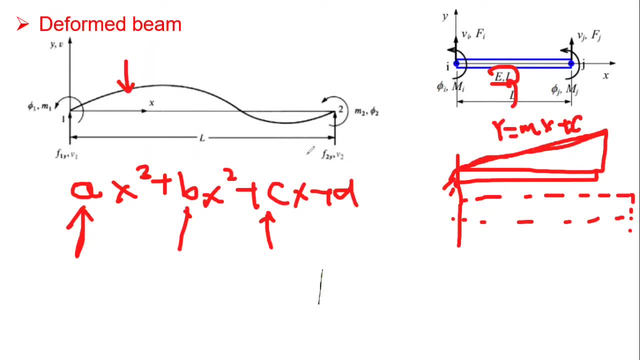 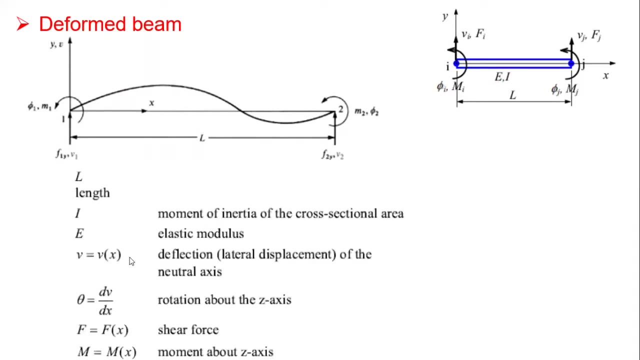 we develop our equation, we express in a matrix form and voila, we're going to have our. our equation: f is equals to k, d and k will be the stiffness in matrix. so v in this term, some uh expression. this is just a repeat of what is in in lesson number. 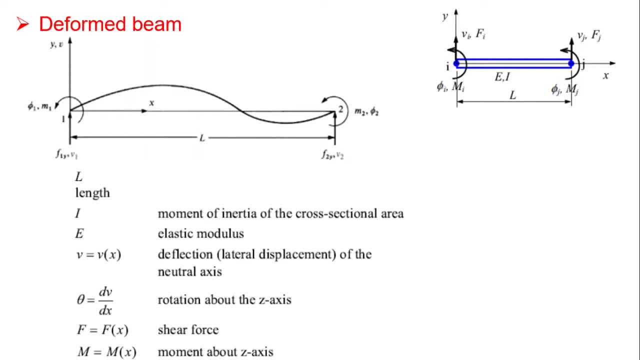 i believe this is a number four, or the beam element about the, the, the notations, right of course, there is the line that is 160, of inertia is elastic modulus, and then v, the component v here is different as v, x, because it's going to find. so you're saying we have a function of x. it's very different from x. 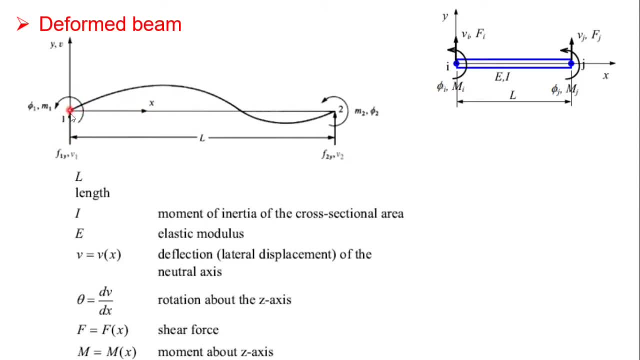 is a function of x, its value is different from. x is in a distance from, and that is the of the independent function of arri蓜 form. X is any distance from this initial node. So this is the x axis, this y axis up, x axis horizontal. this is the origin. 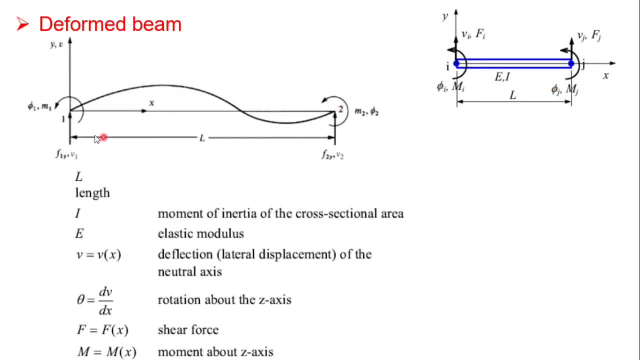 So any distance, of course, up to the maximum here, to the second node x is equal to L. At this node x is equal to zero. So that's why we are saying V is equals Vx. Deflection varies with the value x. distance from the support. Again, rotation. 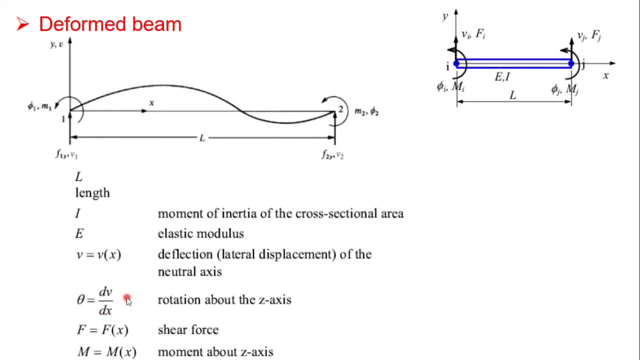 theta, which is the same as dv, the first derivative of the diffraction, vertical diffraction. This is rotation about the z axis, F and M. these are the node of external quantities, These are the shear force which will be the 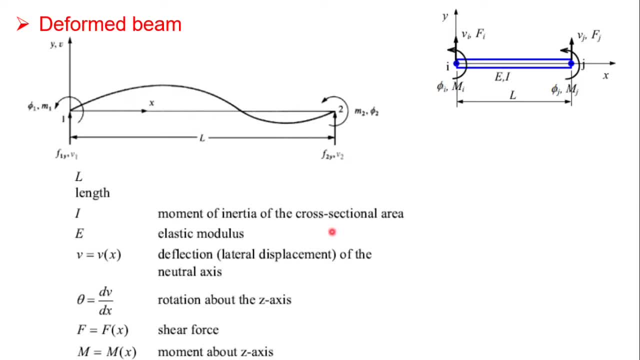 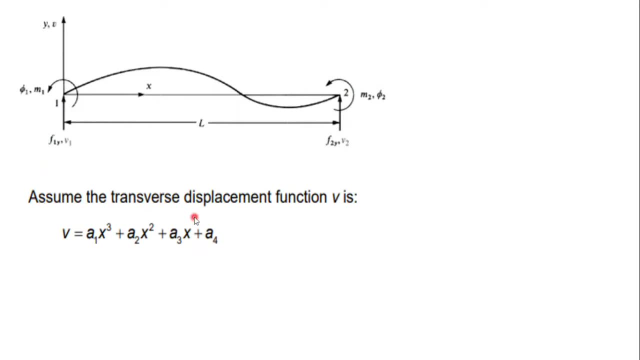 reaction and the moment about the z axis. So just a reminder of that. Then with that we can assume, because of the deflected shape, we can suitably assume that the displacement function V transfers, displacement Transfers, not axiom, Of course. 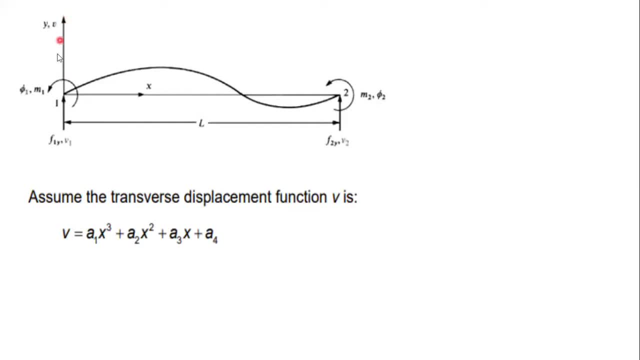 we said for the beam element, we are concerned about the transfers, the load. The load is applied in a transverse direction as opposed to the bar element which was in the actual direction. So the transverse displacement at any point, let's say at this x is. 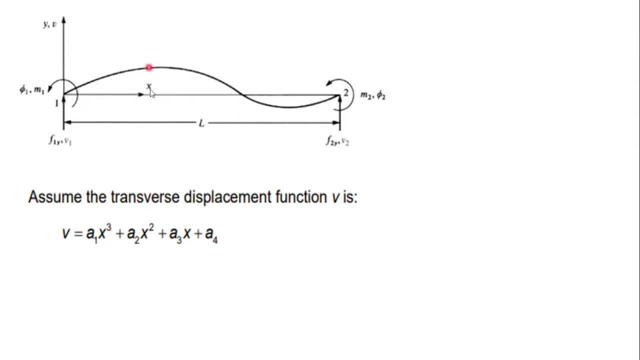 equal to maybe L of a, 4.. So we are talking of these transfers, displacement, here. We are talking of this distance here. Okay, So this is V, V at this location. So it can be expressed as a polynomial in that order, that order. polynomial So: x, cube. 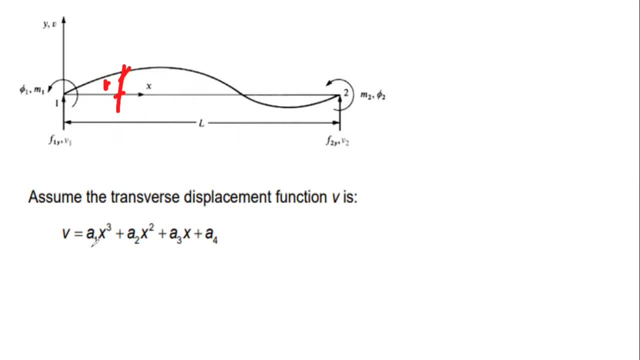 plus a, a2, x squared a3, like that. So we need to calculate or to evaluate. what are this A? What are these coefficients? What we do first now remember we are following just what we derived for the environment, So we use. 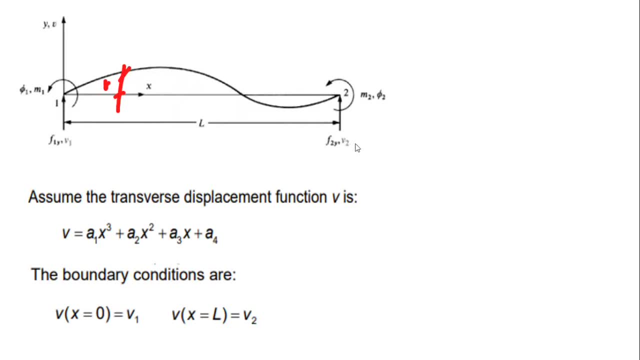 the known we come from. known, First, is the boundary condition, what is given And also what is given in terms of the applied forces. So the boundary condition, you know, at the support here, at x is equal to x, naught of course the 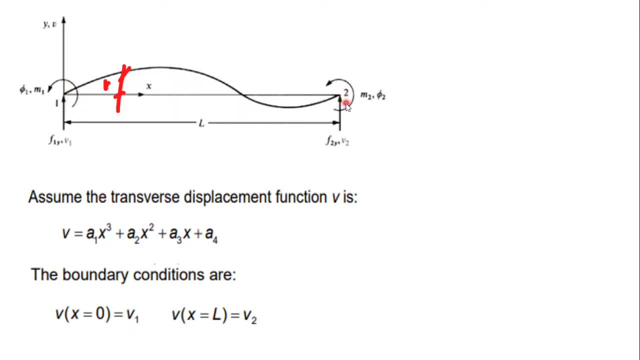 particle displacement, v is equals to v1. and the same case when x is equals to l or, at this support of you, have moved from this origin all the way to this- v is equals to v2. similarly, rotation, uh when x is equals to zero. and remember, notation is uh, the first derivative dv over dx. 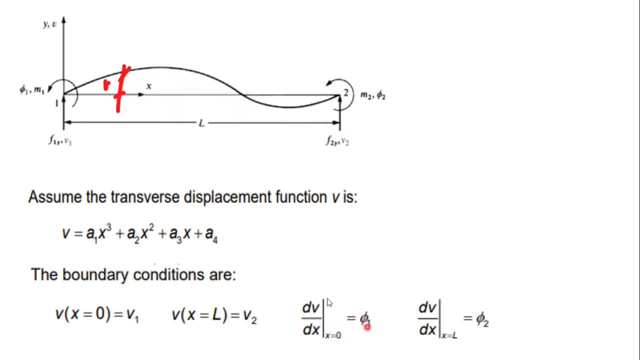 is it goes to: at x is equals to naught, that is, a phi one or pi one, and the dv of radix at x is equals to a direction. here we have v2 and what we are saying is: uh, what this means is that this angle here, this is uh, phi two, you can use it also. and then this angle here, this is five one. okay, 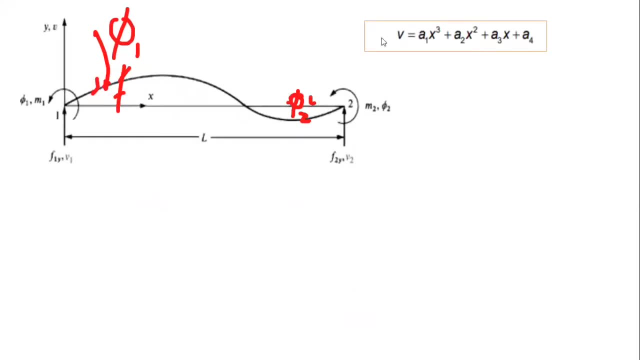 good, what else do you know? so now, this is what we have, and, uh, we have the expression. i put it here. we have our deformed shape. we go now ahead. we apply the boundary condition so that we can solve for the unknown coefficients. now look at this expression: v, the one i've given up there. so when v or when the vertical, 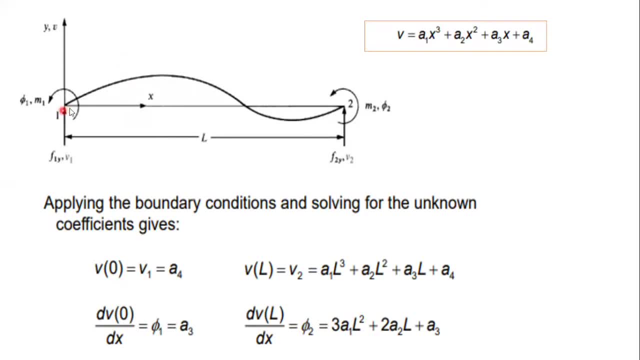 displacement at the initial, the first node here, this node, here the first node, i, or one v, uh, zero. so x is equals to zero. so what we do we substitute in this expression here x is equals to zero. so you're going to have v node or v at zero, v which is equals to v1. all these will collapse. 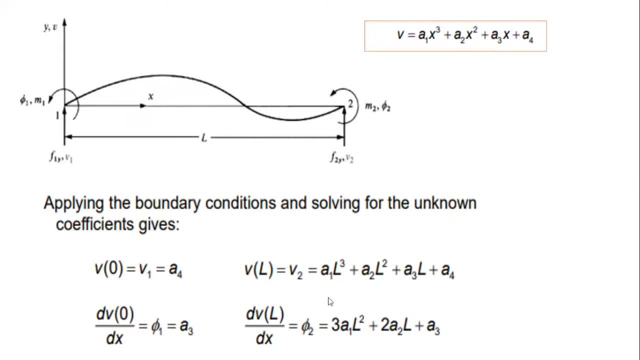 all these quantities here will collapse. okay, these quantities here will collapse because x is equals to zero and if we know that v1, which is v at zero, is equals to a4, and similarly when x is equals to l at this node, so we substitute l, x for l, so you're going to have a1- l cubed like that. 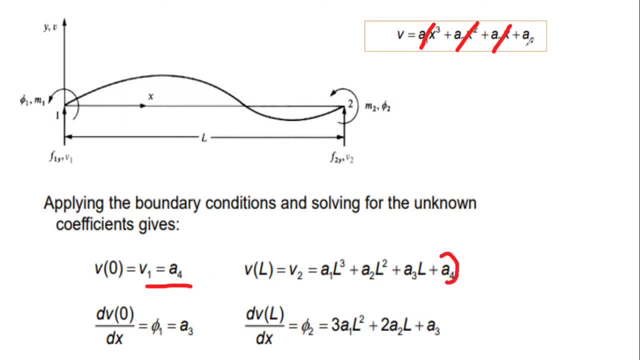 of course we know a4 is equals to. i mean, uh, from the here a4, here a4 is equals to v1. again we move to the second, the component of what is unknown, the degree of freedom, what is known, the rotation at the first node, theta one which is equals to. so what you do to get rotation from this expression? we? 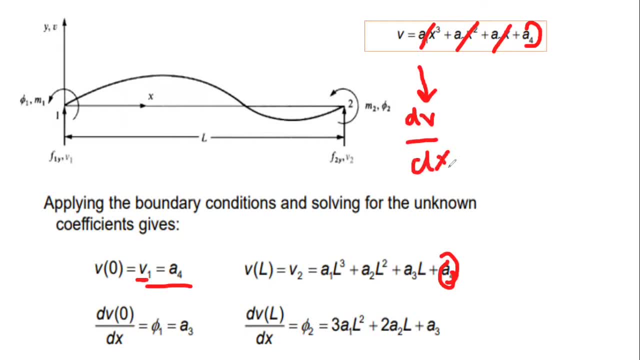 know rotation is dv over dx, so we need to derive this. i mean to find the derivative of this. so this will be three a1, x squared plus two a2, uh, x plus a3. okay, of course this one crosses when you. you find the first derivative. now with this you just need to substitute to get at when l or when x is. 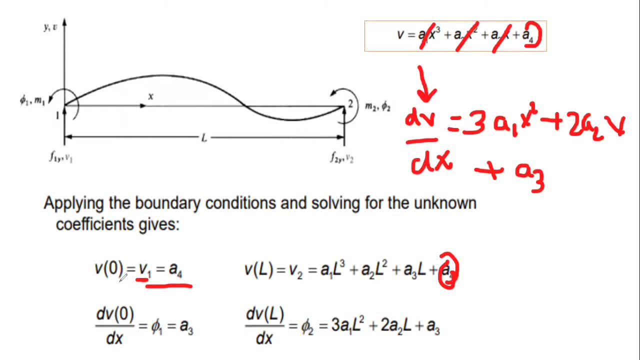 equals to zero at this origin. you know theta one. we want to get beta one, so we substitute here: x is equals to zero, so you are going to be left with this quantity here. so theta one or theta when l is equal- okay, we are using phi, not theta phi one. when x is equals to zero. 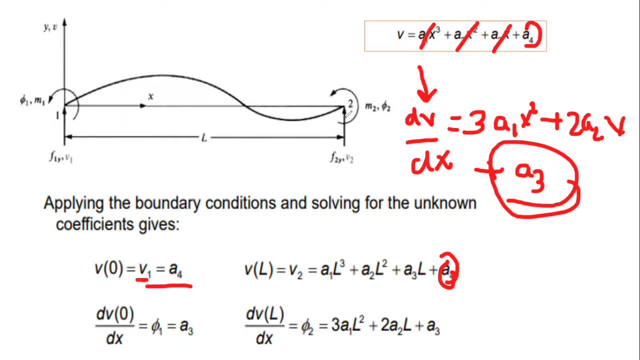 then, is equals to a3 and there, similarly, to get a phi at this, uh, second node, we just need to substitute x in this, our derived equation, when x is equals to l, and then we also approaching fran's equation in this moment, and of course we are using 5-s. cast the Africans. 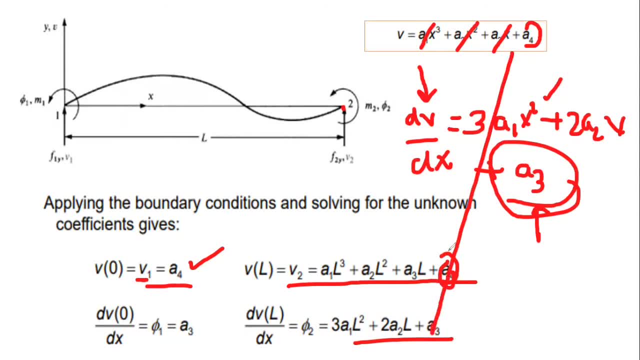 they are going to be through a3, because we know a0-4-s or we know a three. this is data. so you see, we have been able now to express uh using v's and theta, the known value. we have again reduced our equation slightly from what was the original equation here, so we can go further ahead. 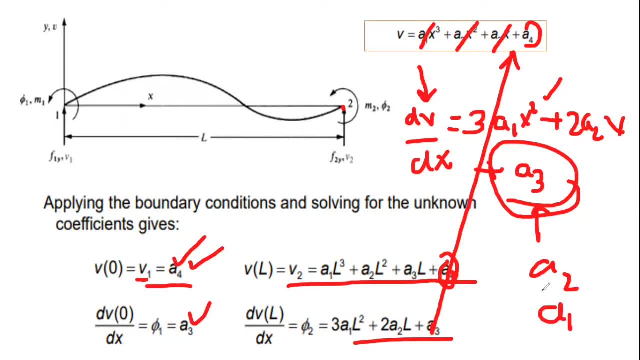 and start now rearranging these equations that we have already. we have: a4 is known as v1, a3 is phi1. make a2 and a1 a subject of the formula in either of these, and then you substitute with the known values of alpha, a coefficient, a3 and a4, so that now we will be left with: uh, we have the expression. 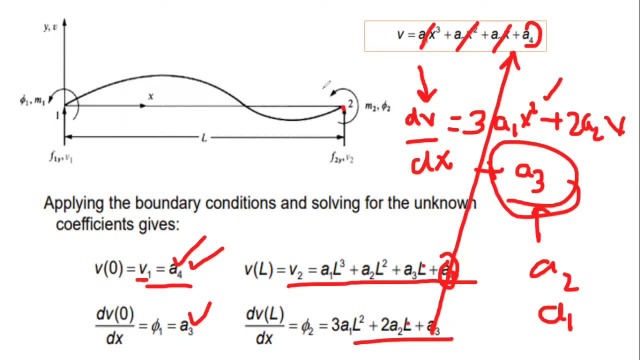 for a1 and a2 in terms of what is known, which is known as v1, theta 1 and l and ei. okay, so let's see what happens next when you do that. so, when we do that, we solve this equation for a1, a2 and a3. 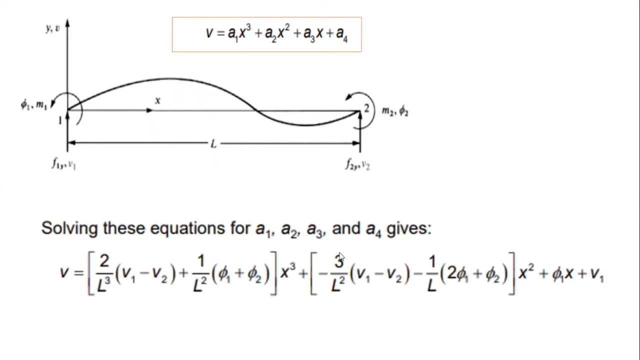 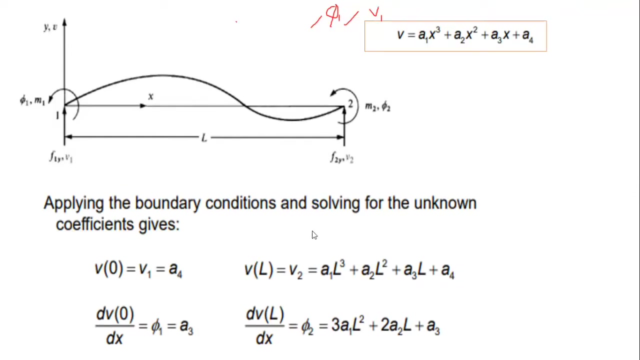 and uh, from our expression here, from our equation here. so this is the equation: we find that, um, this equation, we already have found that a4- this is v1, a3- this is phi one. is it that's true? okay, confirm what we derived: a4 is v1, a3 is equals to phi one and, of course, we have this. 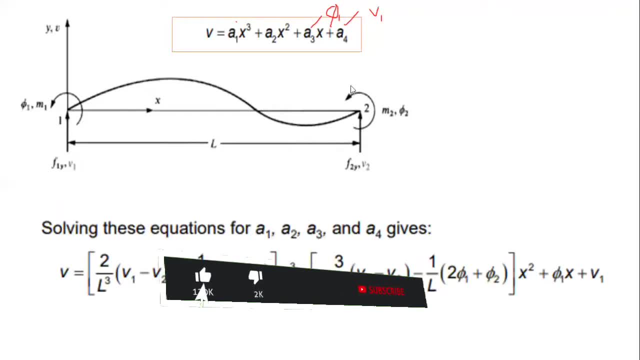 component. so, from rearranging and obtaining what is uh a2, we express it in terms of uh, the known quantities that we are able to see directly in this expression. of course i've jumped some steps here, because it's directly been able to obtain what is this? what's the a4? this is this quantity. 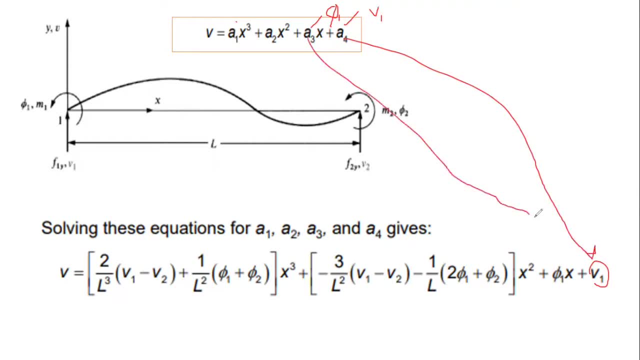 here, then the A3. is this quantity here? okay, So then this part, the coefficient for X squared, this is A2.. And this part, the coefficient for X cubed, this is A1.. And I believe this should not be a big task. 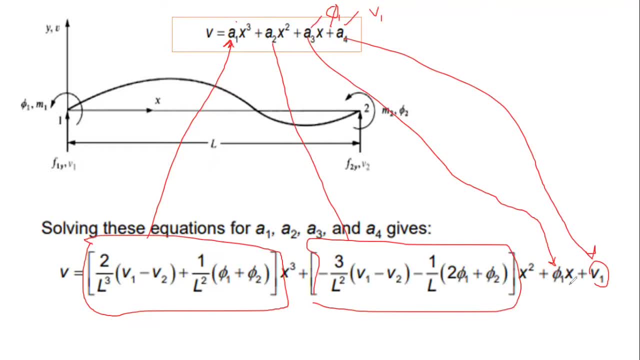 a big handle to obtain that. eh. Yeah. so you see for the first one, what you just need to do from what we derived in the previous slide. eh, It's just you express A2.. Of course, it will have you use the substitution, eh. 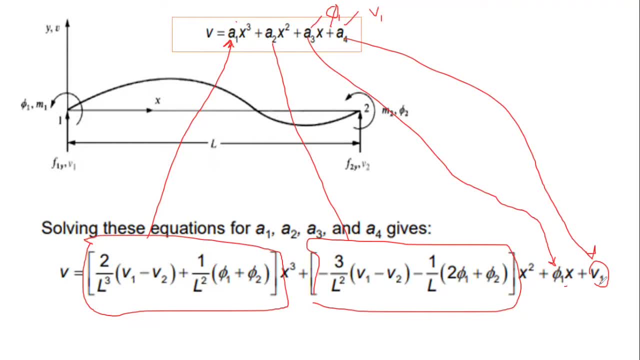 You substitute for the known node of values eta1 and v1, eta2 and v2.. So evaluate that. let me see if there is a there is any need for further explanation on this one, then you can leave a comment, then you can look at it. 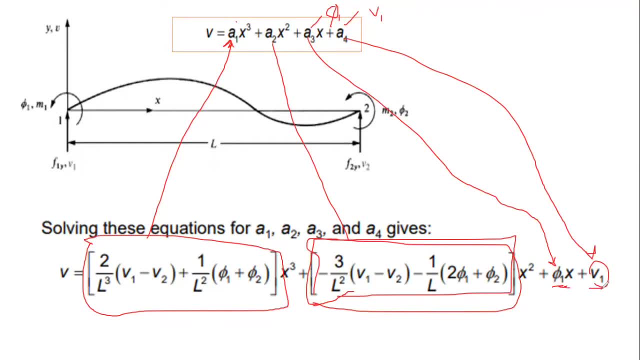 but it should be easy, it should be very easy, Just the same way we derived this like this: So we have the expression for V: V in terms of this is the displacement function. So it means this displacement function at any one point. eh. 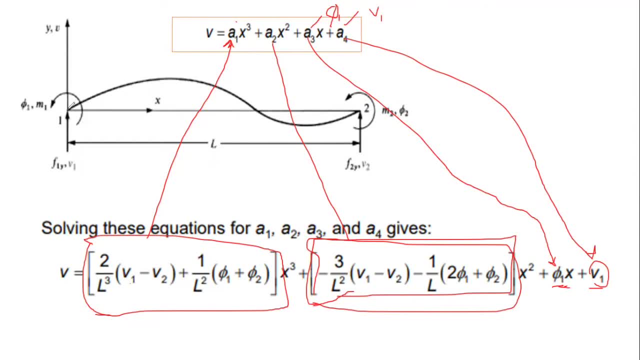 Because we know what is v1 and v2, we know what is the displacement at the node. we have the node of values. we have expressed our displacement function in terms of the node of unknowns, node of values. eh. So we can, once we get these values at the node, eh. 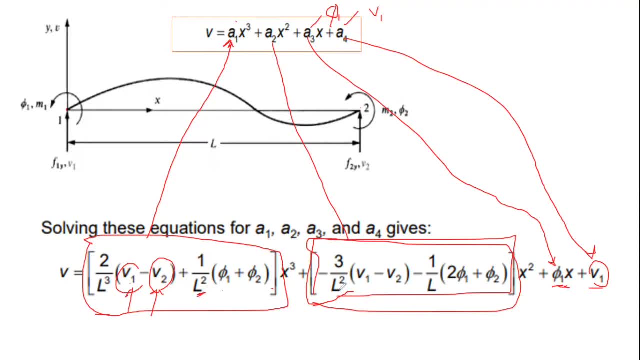 And of course we have this distance. we can be, we can be able to get or to interpolate the displacement between the node at any point. okay, So now, before we move to the next step here we are going to look at: 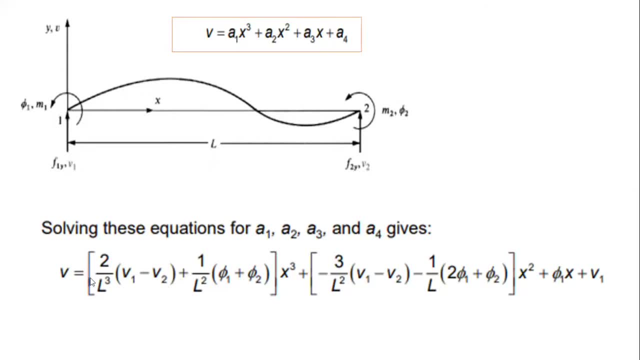 this is now that we are going to rearrange You. if, as you can see, this expression is arrayed in terms of, of course, as a polynomial, starting from, of course, the x cubed, x, squared x, then 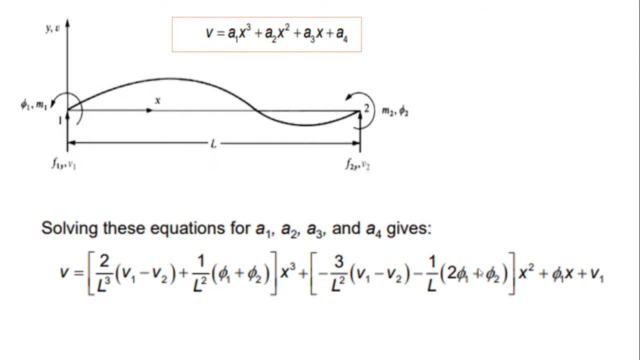 up to when x raised to power zero. okay, We can rearrange. we can rearrange our expression so that we have, in terms of v's and theta's, v1, zeta 1, v2, theta 2.. 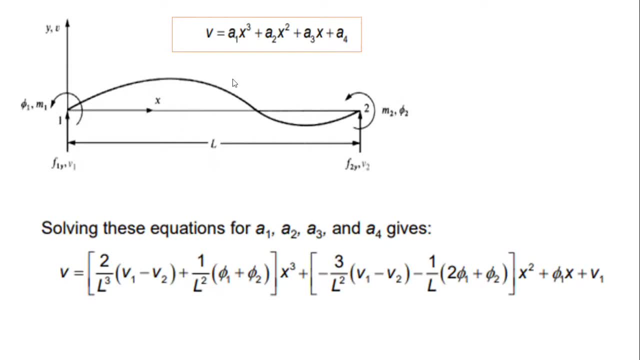 So we just need to rearrange this expression And we are going to see why. because we know from our previous knowledge on finite elements, a method that the examples we have So previously in the bus and all that- eh, We are going to have a vector, okay, 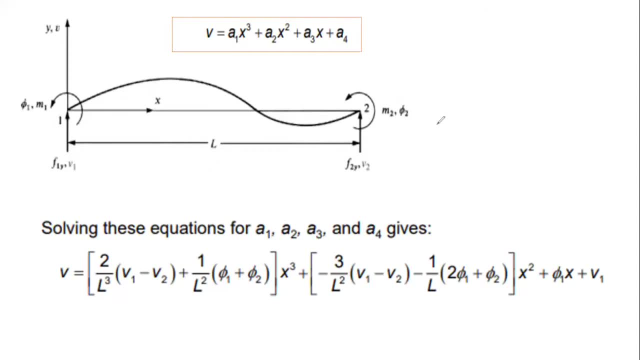 A force vector or a displacement vector. So we are going to have: f is equal to kd And this one we express them. of course we talk from node one. So maybe if f1, f2.. And in the case whereby we have at a node, 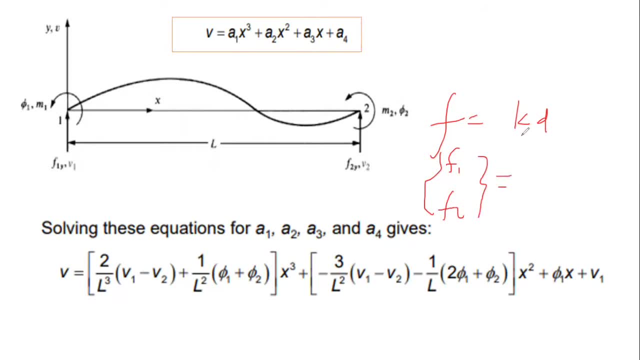 we have maybe two degrees of freedom We are going to have if we have f and moments. now, moments have been introduced, So we shall be having f1, m1, f2, at m2, okay. Same case for the displacement component. 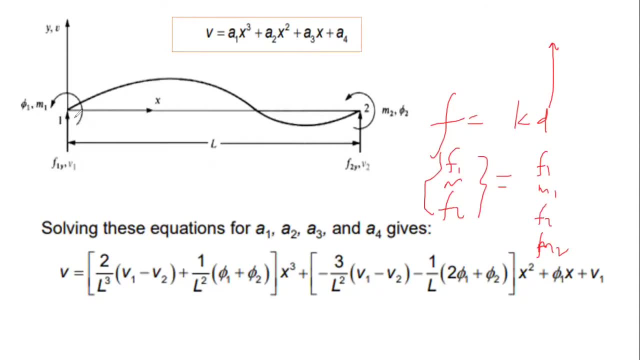 The degree of freedom at each node is theta and v- small v- okay. So you're going to have v1, theta 1, v2, theta 2, okay, As the displacement component. So that's why it's wise. 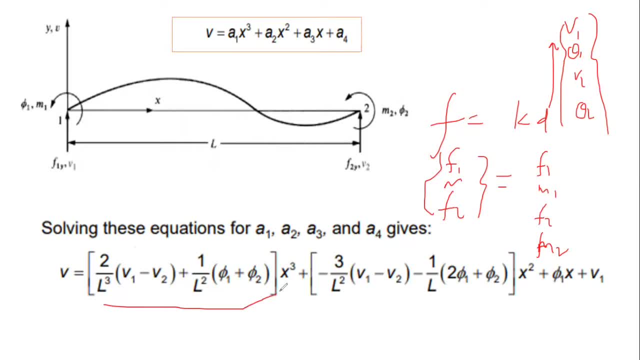 Because you can see v1, v2, they are together in one. You know we have made like this v as a function of x, So we can rearrange it and by so doing, because you know our end-product. 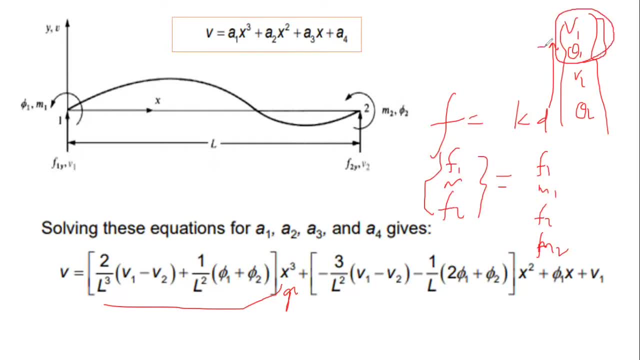 our end-equation will be in terms of node quantities, node one and node two. okay, We can separate that, And this is what is done in the second slide and this next slide here, That this rearrangement. I have rearranged this one here. 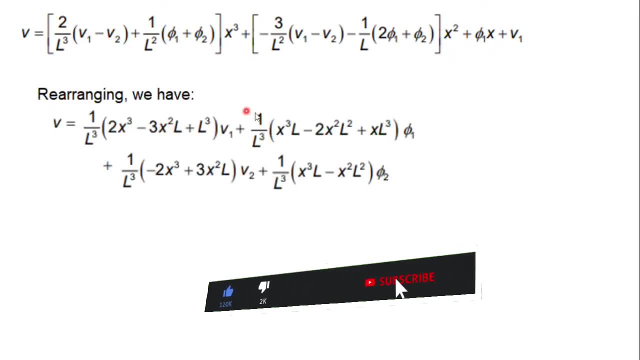 This is the equation that we have. Then this is the금. Okay, rearrange equation so that we start with v1, theta 1, v2, theta 2.. so to rearrange this, you just need to open the brackets. so you open the brackets here and then. 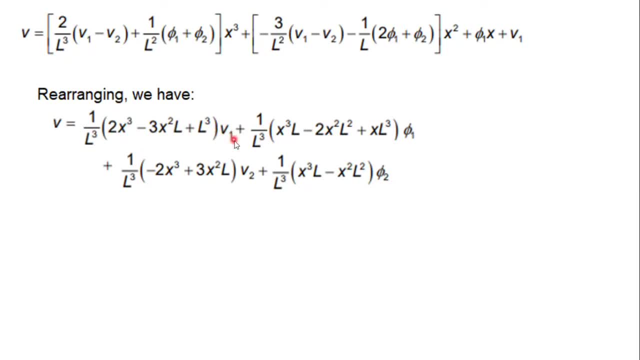 you bring the common terms together, the common terms that have got v1, those that are got phi 1, v2, phi 2. okay, so you know now this one you can be able to write in matrix form and then at the end here you have v1, theta 1, v2, theta 2.. 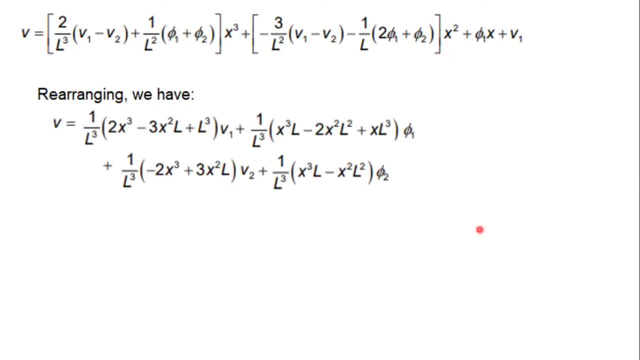 that's the purpose of the, the motivation for rearranging now. with that, now, we move to the next stage, whereby, of course, before we move to the next stage by rearranging like this, remember we talked of, uh, what we call the, uh, the, the shape function, okay, the shape function. and we said: 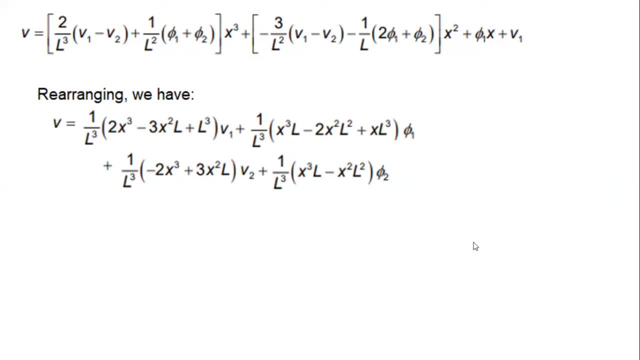 for the shape function, which are kind of the interpolating function that we use and i remember very well we derived for the bar element and we say the shape function. these are the assumed shape of the displacement field within the element through the interpolation of nodal displacement and 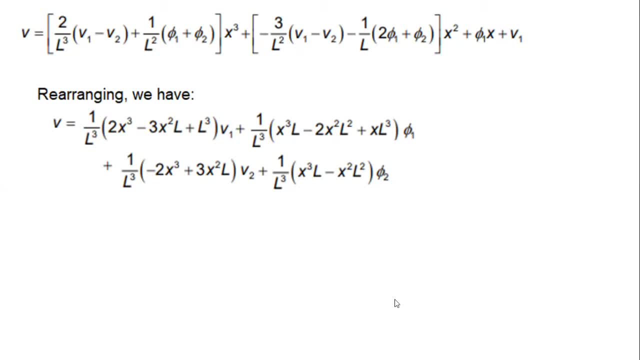 we had for the bar element. i use this so that you can refresh. we we had two cases for the bar element. it was like that we have to shape function linear. so the first one, which was n1, was equals to one minus x over l. okay. and then the second one was x over. 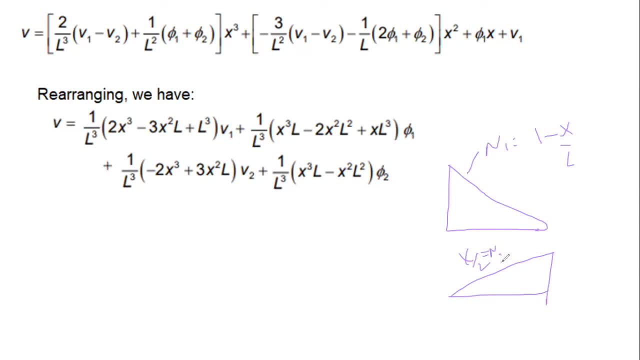 r, which was n2, and uh, this is equals to n2 and because of that, we could be able to simplify our displacement function. we could be able to say: u, x, for the bar element was equals to n1u1 or ui plus n2, uj or u2. okay, so the same case here. we can be able to see the displacement now in this. 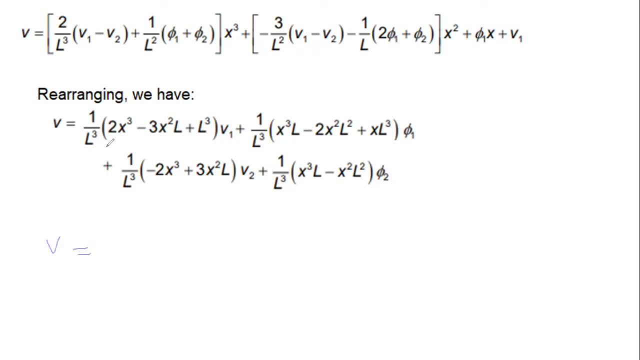 case, division is not: u is v, v is equals to. now this component. here this component is the displacement function. you can say n1, v1 plus n2, v1 plus n3, v2 plus n4, phi of e2. okay, so these are the shape function for a beam element. you can see this is they are quadratic. 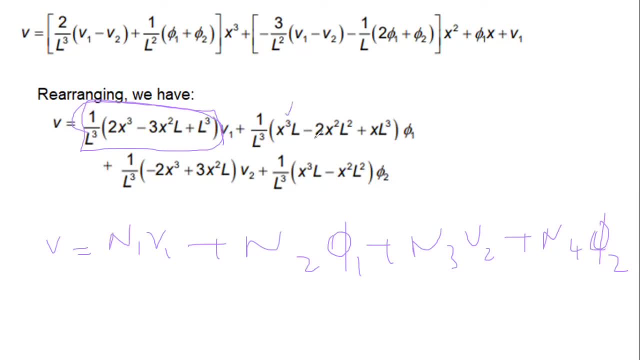 they are cubes, cubic in nature. they are in x, raised to power 3.. so these are the interpreting function of the shape function n1 out to n4, and we can sketch briefly this shape: this is a cubic expression, so you just need you know. the shape function, of course, runs from zero to one. okay. 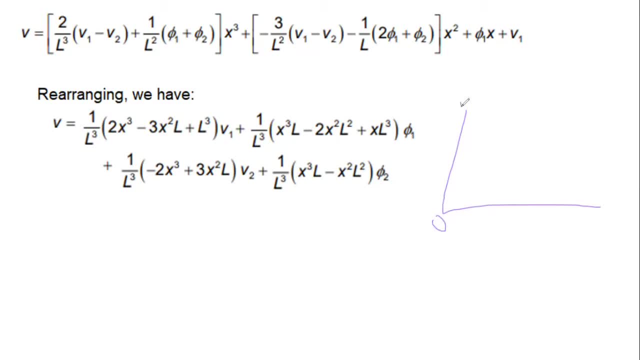 zero to one and neither axis zero to one, so you can substitute to an: x is zero when x is x, x is one and then another values in between, because we can see this is not linear. so at least maybe three points and the typical shape that you are going to obtain, which is the shape 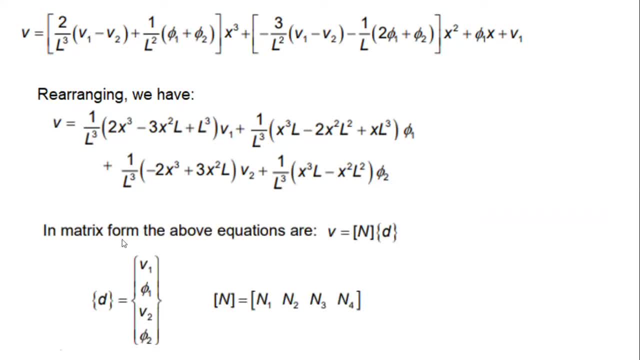 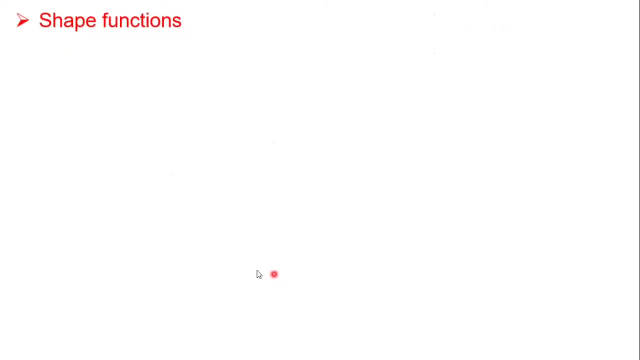 for this shape function is shown in this sketch. of course, this is just explaining that we can be able to use a shape function. we simplify our expression for displacement, displacement function. so v will be n times the for uh, the displacement factor given like that. so this is the typical shapes. 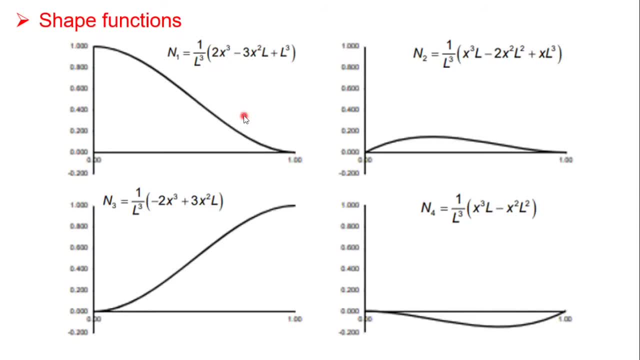 you do not need to come this. maybe you can just look at them and then familiarize yourself with them. the n1- how it will vary- n2, n3 and n4. so these are the typical shape of the uh, of. this shape functions all right. so we are moving on well, and the next thing that you need to do is that uh. 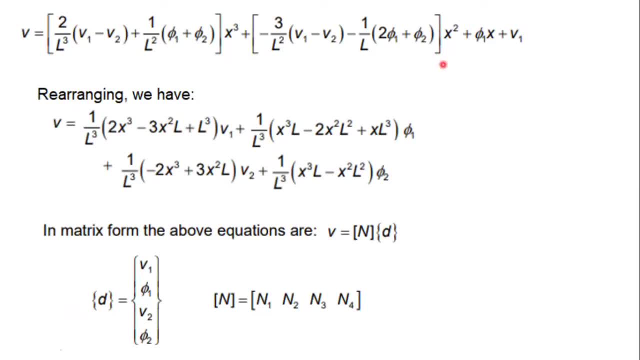 from our derivation. i've gone backward one step so that we can be able to look at these. so if we look at this, uh, the next thing that we need to do to to develop is that we know we need to come up with this kind of an equation: f is equals to k, uh, d or delta and then f. these are. 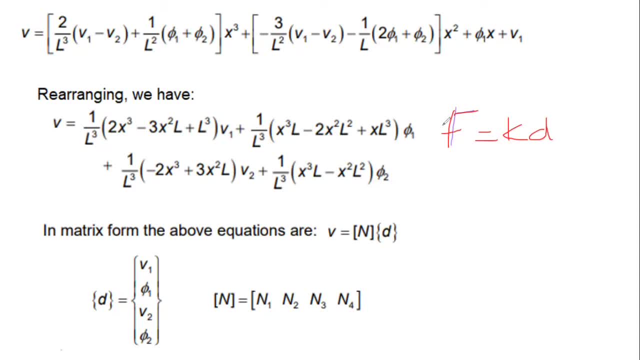 the nodal force or applied loads, nodal load quantities. so i do know, at the node we have forces, so we shall have f1, m1, f2, the second node, m2, forces and moment is equal to the k, because we are still deriving k. then, uh, we have a column vector, for this reason, component, and at this node we have v. 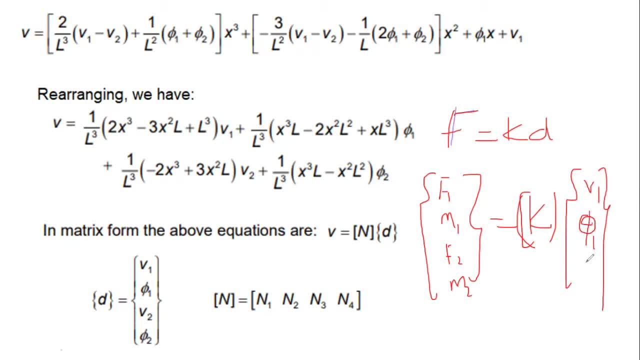 the vertical displacement and and the rotation v1- v1 and the v2- v2. so what we need to do now, because already we have the displacement function, We need to use this displacement function and the theory that we know from the previous studies, mechanics and all that we can be able to get. what is the expression for the? 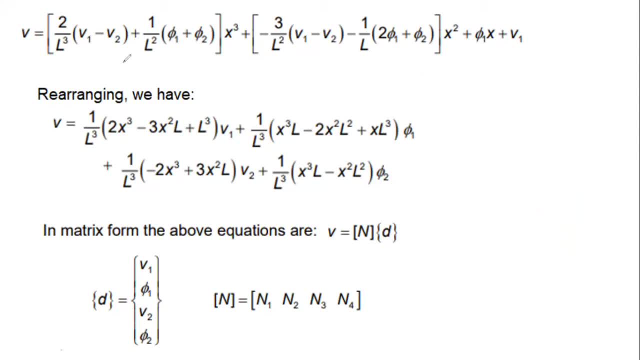 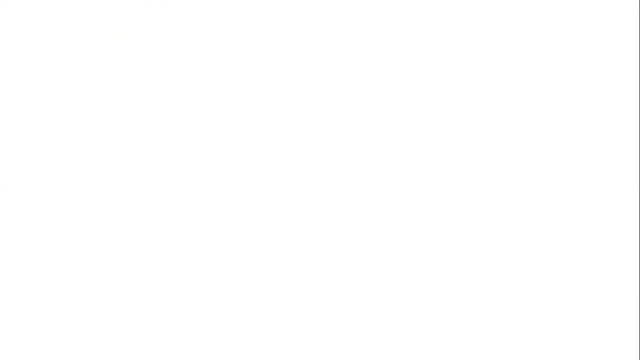 moment in terms of the displacement, And to do this we need to employ a little bit of the beam theory, And from the beam theory there are a few notations or a few things that we can highlight here that you maybe as a reminder, because you studied this in your undergraduate maybe. 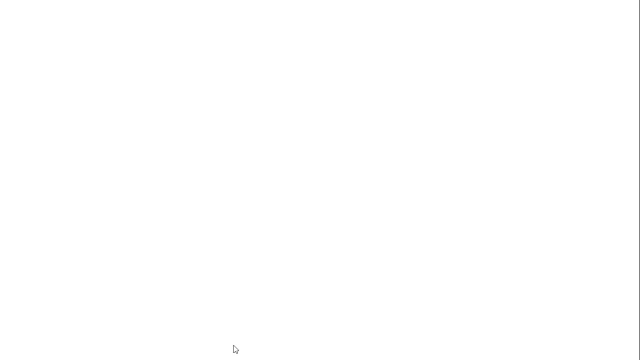 early stages there and you learned about in the strength of materials or in theory of structures earlier on and you had some expression for the curvature You could start from, let's say from curvature. a diffraction, sorry, a diffraction could. 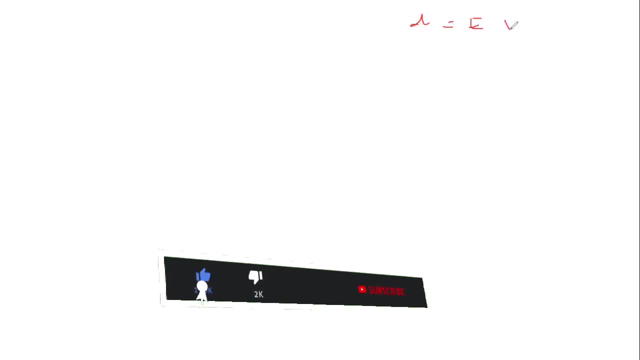 be given by which is equal to. now you introduce V, Diffraction, of course, is V, So you introduce the rigidity, Because there is a diffraction. There is a diffraction, So the V that we have given, the equation for V, that is the displacement function. 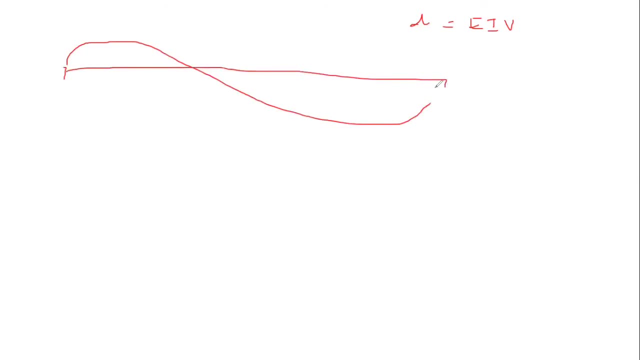 But depending with which material, you could have a beam, a beam which is made of steel, You could have a concrete beam. So we know the magnitude, of course, will be a function of this displacement function, as well as the rigidity. 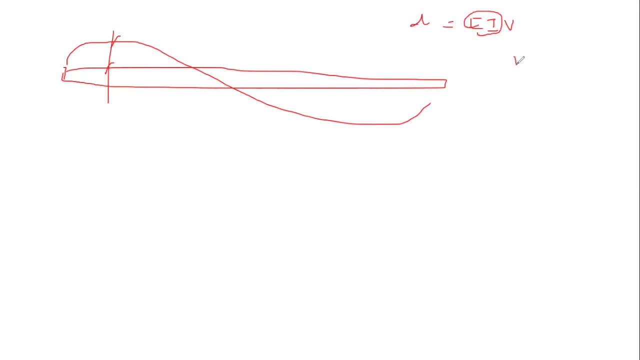 And that's why we introduce the rigidity here, So for the diffraction. so we say V, we express, as we bring in the rigidity and then the function Vx, what you brought about there. Then from V we have the slope or rotation. you know the slope or rotation, of course. 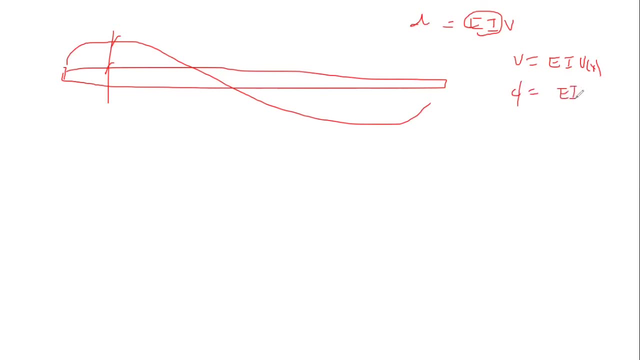 now you bring the same. Of course, EI now will continue to represent the material characteristic and the geometry aspect. So this is the first derivative of V, dV over dx. Then we have the moment M is given by now, the second derivative. 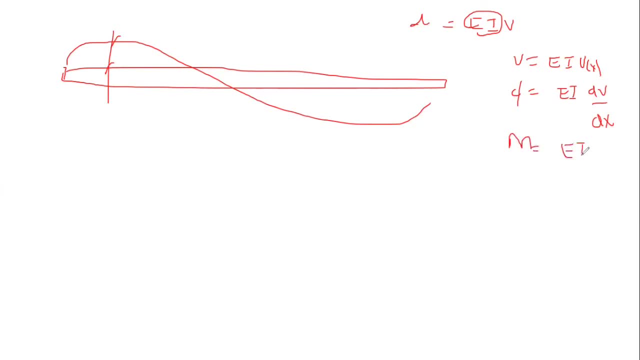 This just reminds us of the moment, So the moment M is given by now. the second derivative: This just reminds us of the moment, So the moment M is given by the new of the area nodes. So, d squared, V over dx squared. 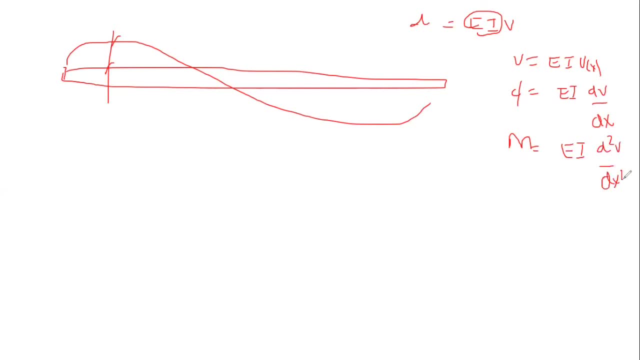 Then the shear force, capital V. the represent shear force by capital V. this is the third derivative. so AI equal to d cubed, v small v for displacement over dx cubed. And finally, we know for UDL, uniformly distributed load and size, that D x is equal to Vx. 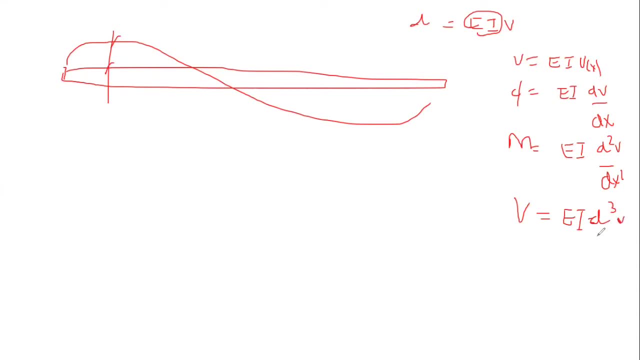 So this is the derivative of the moment. So the moment M is given from V, that D x is equal to v, so that D x is equal to Vx. So that's for us Good. And now we go back to what we call the active momentum. 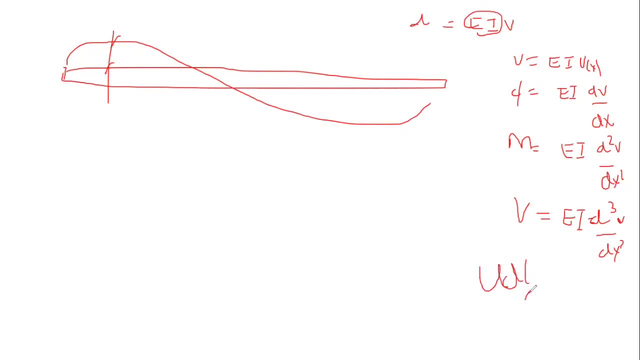 So we are given the linear momentum of the moment. We have the velocity. this is the input static velocity load. okay, which is sometimes represented by, of course, w is the fourth derivative. all that relates to power four. v over dv is to power four. so these are just. 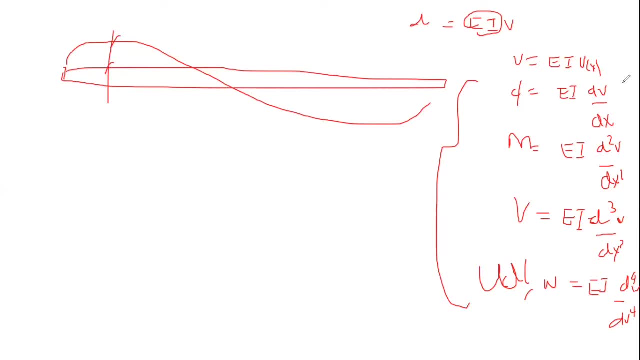 some important expression: you like a land area? no, these have been brought together from different, uh different- lessons that you have covered previously and in our case, here we need to improve. we just need to employ this because we know our nodal quantities of the applied nodal load is only moment under. 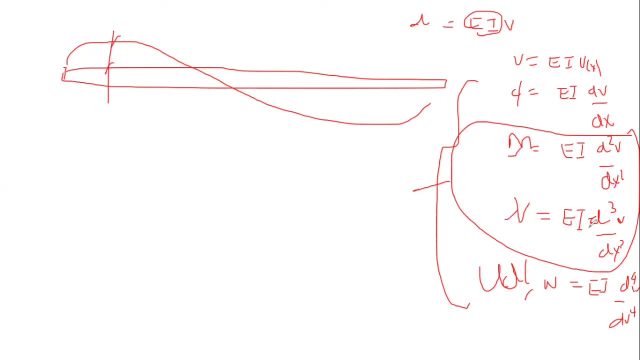 shear force or the lateral force, v. so we need to get the second derivative of a displacement function and the third derivative. okay, again something else also we need to introduce here: when you are deriving this, remember the, the notation upward for shear forces and loads, the beam theory and also 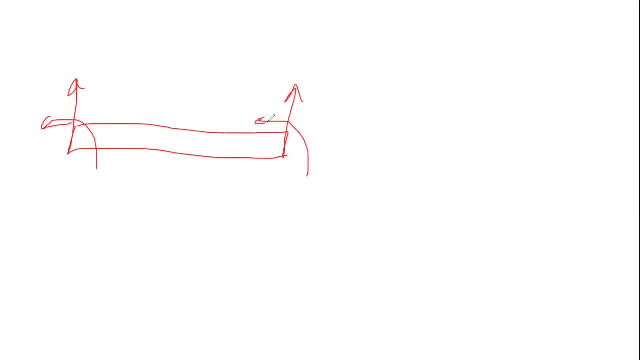 the moment are counterclockwise. okay, and the same case with the fetus. now we bring in the beam theory, because now we are using the expressions from the beam theory, so we know the shear forces. they are positive in the clockwise direction, so in this direction there's 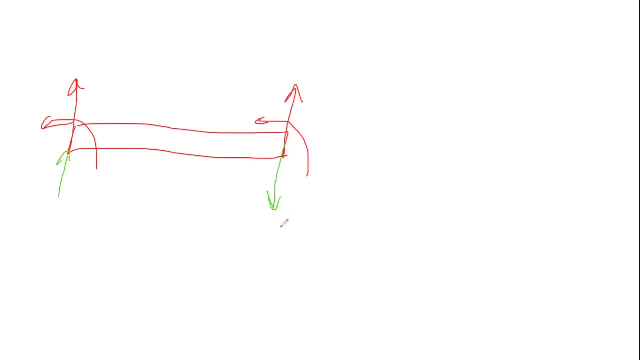 the positive shear force in the beam theory, this one will be downwards and uh, similarly for the, uh bedding moment. we know that uh, the, the, they use the counter, the hogging and the sagging moment aspect. yeah, okay, so that in our case here, what we need to look at of what we know, 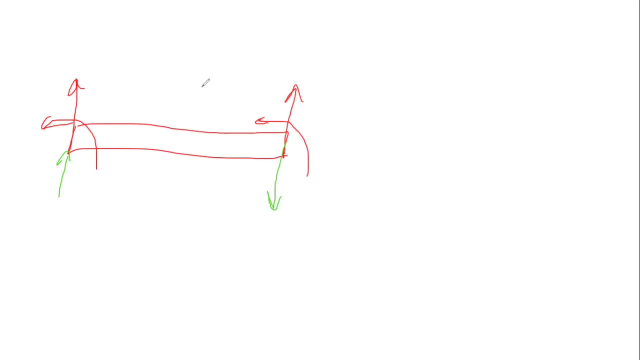 maybe i can project this so that you can start what i'm saying. so this is what i'm saying. you are going to employ these expressions, so i was giving you a reminder of what you already know, so that we know from where now we are extracting this. 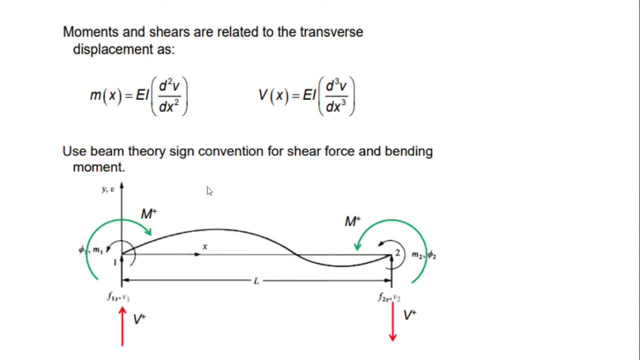 so from the beam theory, we have that. so the beam sign convention, this is what i'm saying here. so we have these. uh, the the one in red at the green are the beam theory, the one, of course, previous slide that i've shown, designed blacks, so you can see there are those which are positive. 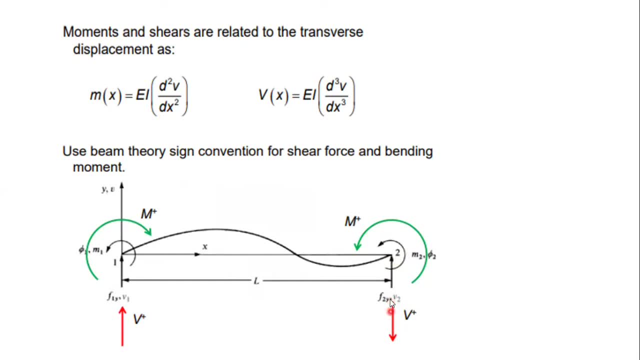 and then those which are negative. if we consider, for example, on this end, node 2, the shear force for the beam theory is downward. so whatever we obtained, our shear force is upward, the quantity we are calculating, so it will be negative v in the beam theory. so the same case with the moment. 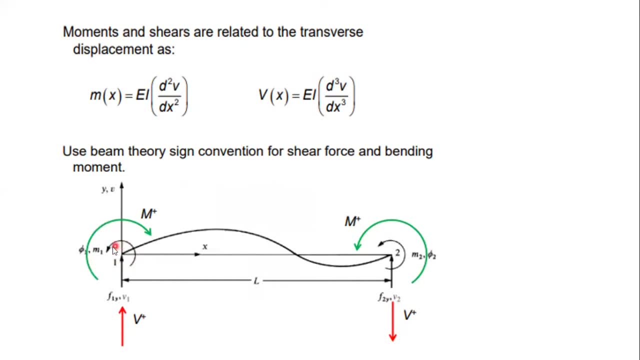 at node one. it's opposite of what for the finite element, beam m1 is, is possible. so because, uh, hogging moment positive, we consider positive cases. so the size, the sorry, the sagging moment will be concave on top one. so that's why now we have the positive moment, so not here. that 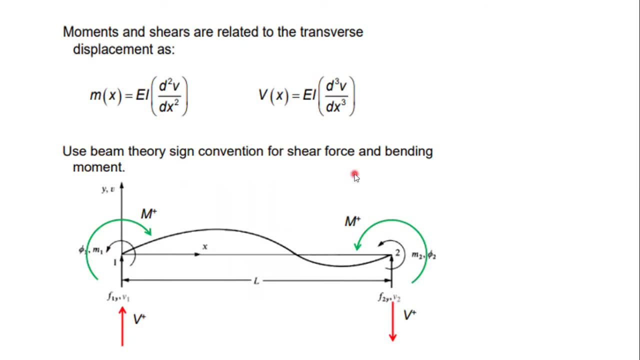 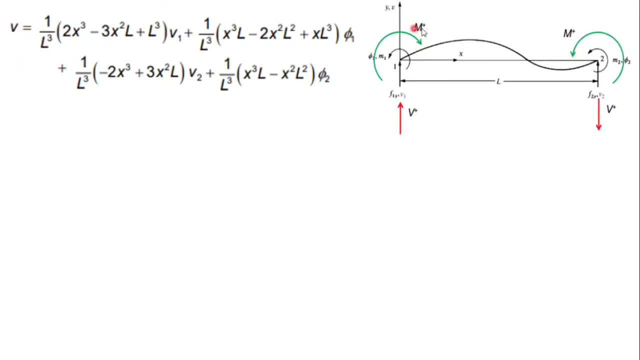 we are bringing in the use of the beam theory, the sign. this will be affect the sign of our expression. so now we go ahead. this is the expression for the displacement, this is the sign convention. so we we need to get what is f, the first f, right with that derivative and the and. 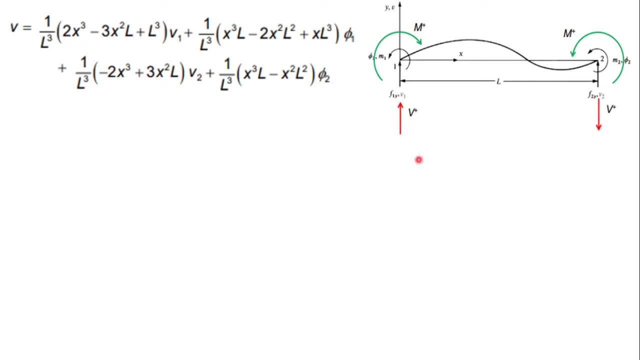 the and the, the second of that second, for the moment, that for the for the beam, and we can start with the first one, f, which is the shear force here, the shear force at this node, capital v, of course, dv cubed over dx. okay, remember the two, the two expression that we are using for the v, for the. 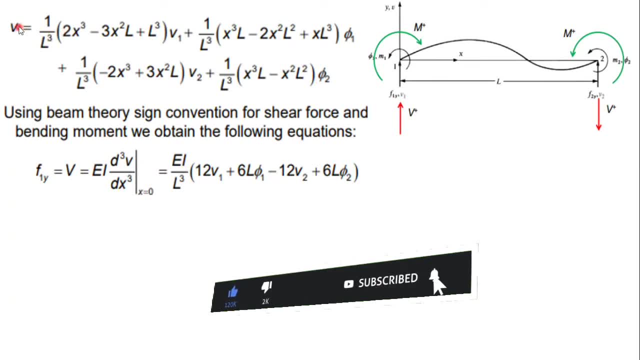 shear force and the heading moment. so what you need to do is that you need to, uh, find a derivative of this expression three times, or the third, and differentiate three times. so the first time that you differentiate, let's just do this for the for the sake of understanding what we are saying. 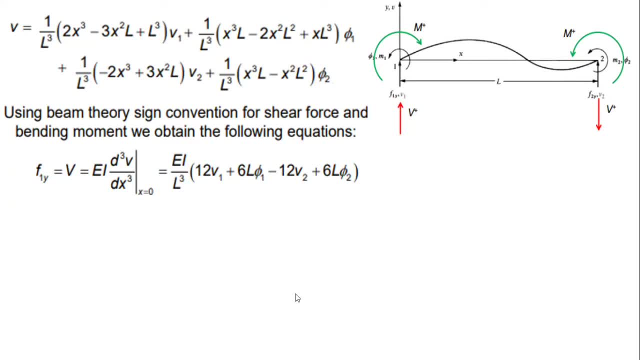 so the first one that we we get here, what we are doing here is that if you that find the derivative, or you you differentiate, the first time here you're going to get, of course, is with respect to x. so you're going to get six uh x squared um, minus six x l, of course, this one now. 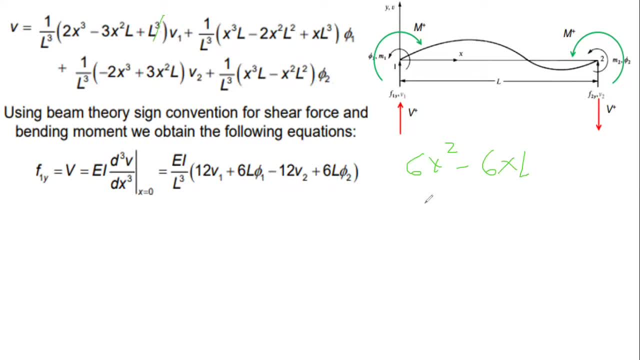 if you differentiate the second time, you have 12 x minus 6 r. if you differentiate at that time, you're going to be left with 12 and this is this component, what is before v1. so all these corrupt system. of course we have taken out the ei and the l cube because it's common l cubed is common for. 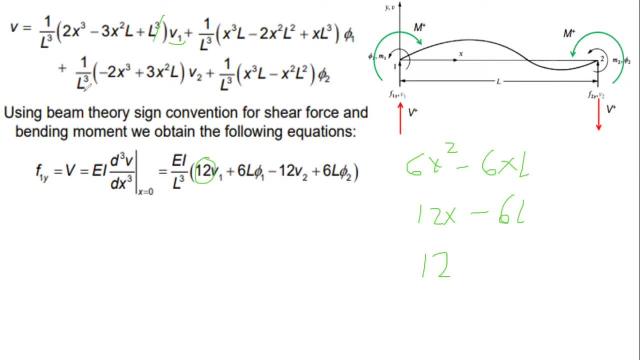 all these, and so you have taken it out. it's a constant. you have taken out. it's here, so you can have. it is a constant, so you have taken it out. it's a constant, so it is a constant. you can find the out. it's here, so it's that way. it's coming below this one. l cubed here. okay, so we differentiate. 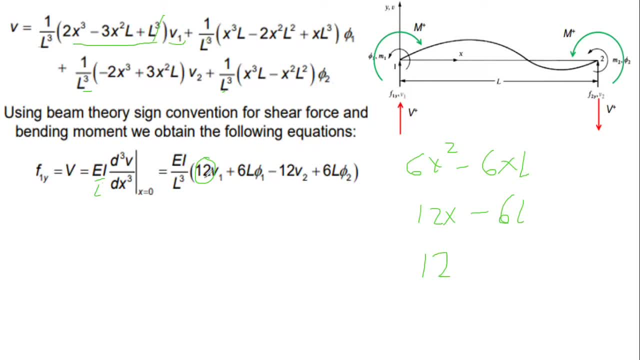 what is inside the bracket here three times and we have seen how we have been able to obtain 12.. same case for this coefficient for phi 1. so the first round you differentiate, you're going to get a 3 x squared l minus 4 x l squared plus l cubed. again, you do it. the second time you're going to be. 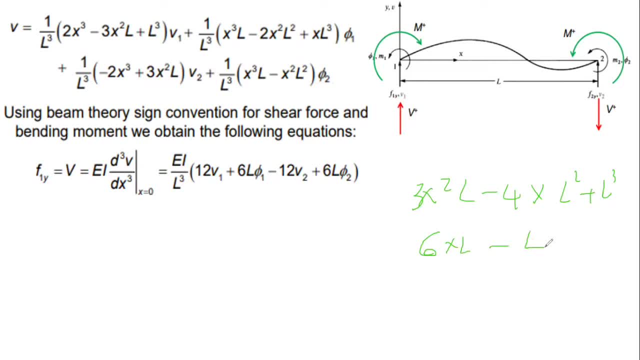 left with 6 x l minus 4 l squared. this one now goes again. the third time you'll be left with 6 l, and this is component here. so you can do the same here and the same here. so this is for a f. f at x is equals to 0, the f1, so you do the same for the moment. moment. you just need to. 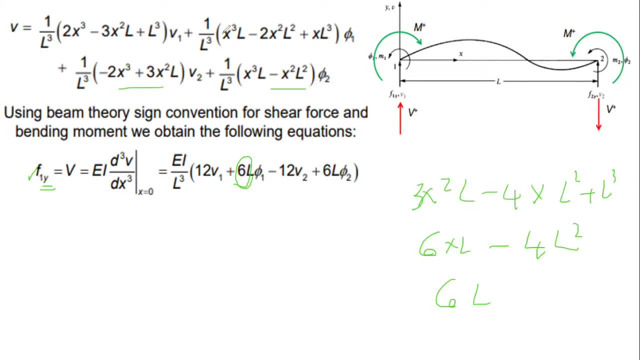 differentiate twice. okay, so you have found how. what you are doing is very easy. you just need to differentiate the this component here twice, and twice for movement and for shear forces, and then with that we can be able to obtain this. so f2 when x is equals to l. okay, so at this head you are differentiated there. 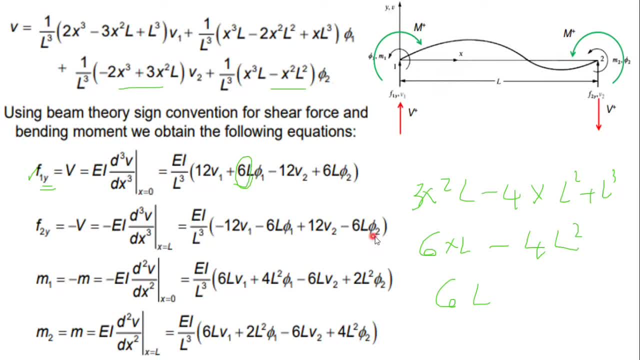 you substitute the values, the known there. so you're going to be left with these expressions. so you can see, i've been able to obtain the shear force at the first node and the second node. at the same time you have been able to obtain the moments. so this is the second derivative for the moment at. 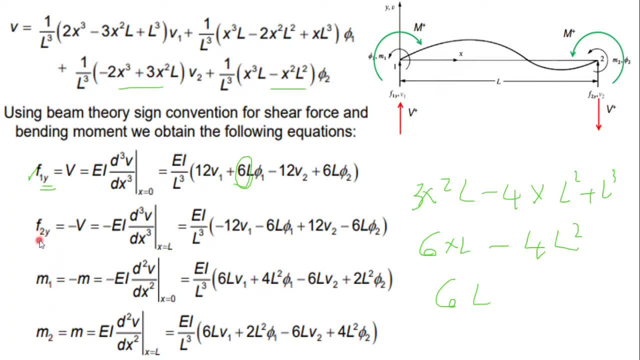 the first node and the second node. so you have f 1, f 2, m, 1, m 2 expressed in terms of v 1, phi 1, v 2, e 2. so looking at this, we know, now we can- uh, we, we are slightly just about to write our expression. 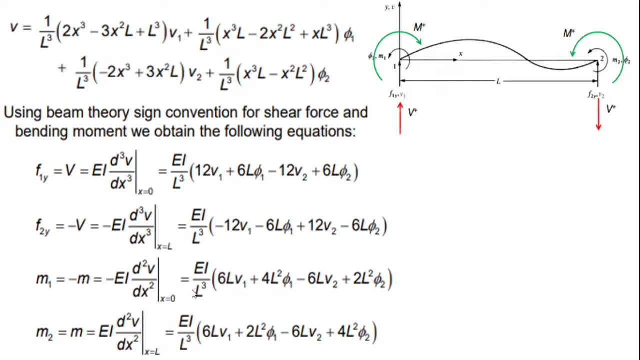 or our equation finite element equation. remember this one have to stick in your mind. we are, we want to come up with. f is equals to k and of course we express the, the expression, other, the quantities from node one that accounts for so v, one, uh v one, phi, one v two. 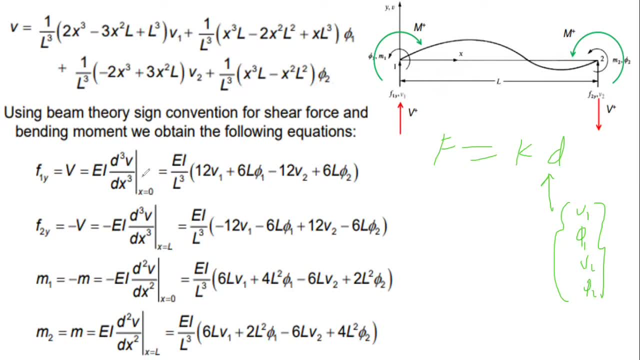 y two. okay. so, looking at this, what this one tells us is that for us to be able to write f1, m1, f2, m2, like this, and then we'll have k, so we need to rearrange this component so that, uh, we'll have the v1. 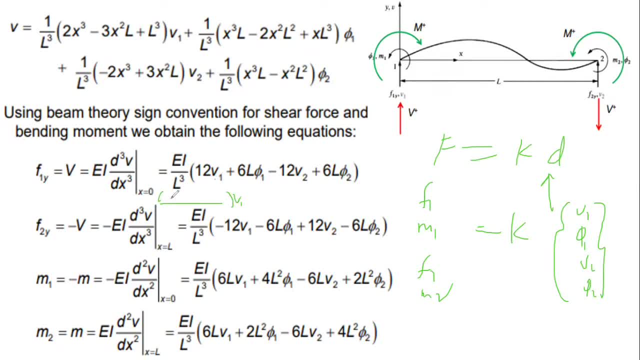 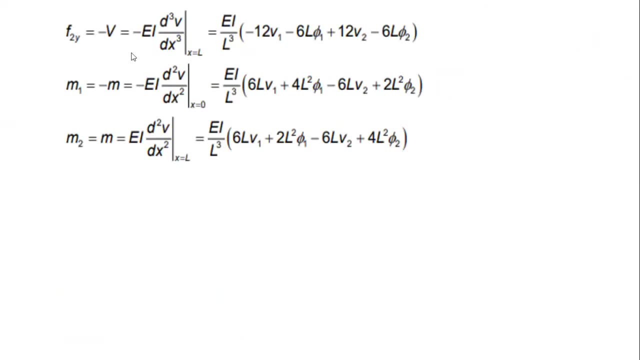 factored out. we have what is the common, what is common with v1, then we have what in bracket plus for the y1 and y2, phi 1 and v2, like that, so that now you can be able to write in matrix form. and this is now what proceeds in the second slide. so this is the writing. let's return, okay. 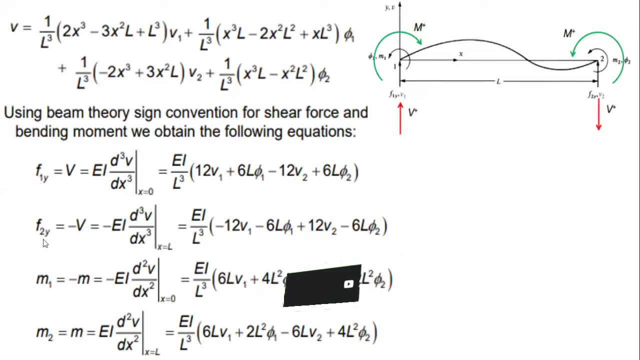 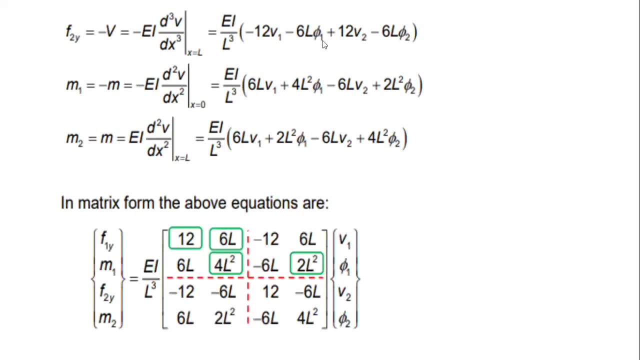 so f1. there is not zone in this slide, so f1 is here. f2, m1, m2. so when you come here writing like that, and therefore in matrix form, you see the v1 starts here. okay, so these have been written. f1 is somewhere out there, not shown, so, but this in essence. that's what we are doing, just make. 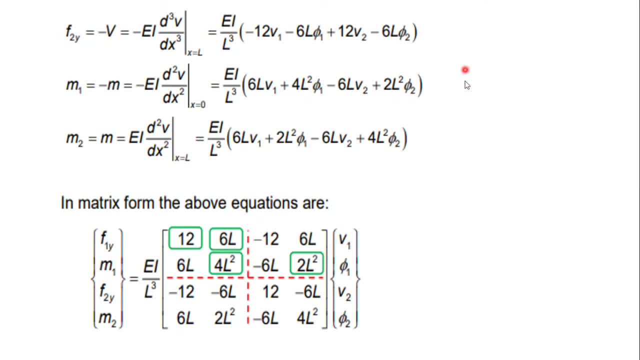 sure that the component for v1 are put together, the component for phi 1 are put together, the component for v2, like so on and so forth, and with that now you'll be able to write in matrix form the equation and uh, from here now we have finished with our derivation, not only for the mass stiffness. 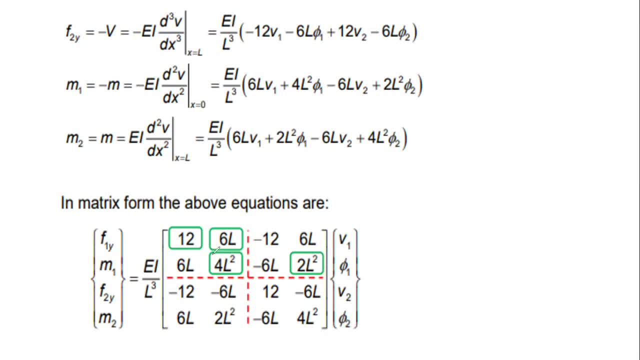 matrix, but, at the same time, we've been able to obtain the finite element equation, because now, this is a value of f, this is k, this is d. okay, so all this is what is the stiffness matrix, what you wanted to derive, and, uh, this is the way that i used to remember this- uh, this stiffness matrix. 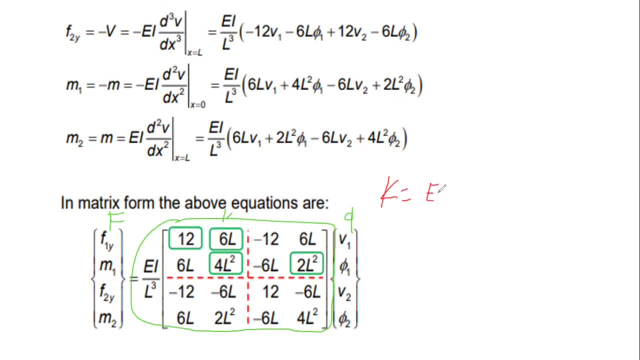 maybe is a an addition. k is, of course. i know there's ei of l cubed out there, then inside, here we partition. that's why i'm using the headline. this is the way you can use to remind you a second. so just need to remember that is 12, 6 l, 6 l, 4 l squared. okay, that's the only one, that's. 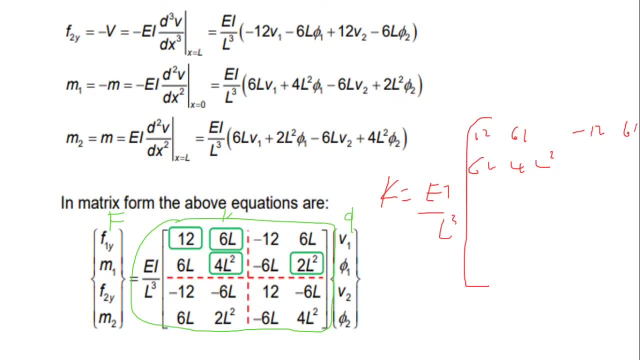 different. and this one minus 12, 6 l, minus 6 l, 2 f squared. so there's the rest. i know this one, i take it here and i put negatives in the minor diagonal. now this one, i bring it here and i interchange the column or downwards, then the negatives will be horizontal. so i just need to remember this and 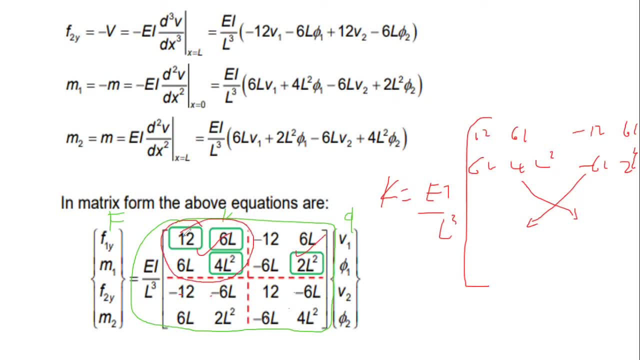 this, and actually you just need to remember the first one. okay, the second one, you know. the only thing that changes is that this four is two here. so what happens in this case? we have the negatives introduced, this becomes two. so anyway, that's neither here nor there, just a simple way of how. 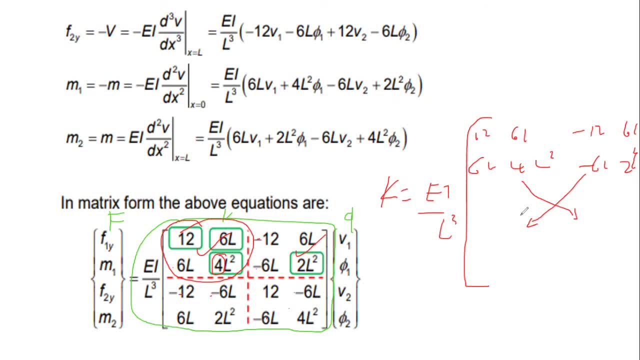 you can remember this, but again, it's not a matter of crowning. if it's in an exam setup, maybe i think you should be given this one as a as a reference. okay, that's all for today. if there's any question, leave in the comments section and, uh, let me know how these lessons are. are helping you. 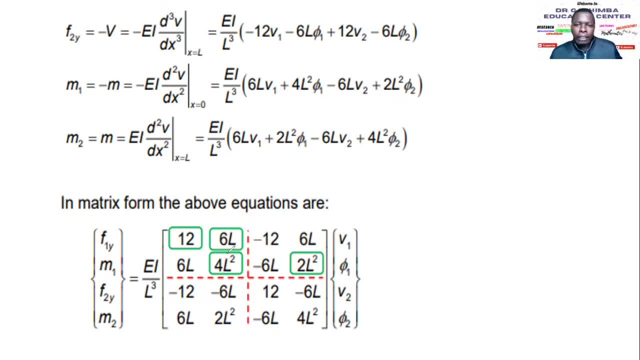 and uh again. if you have never uh subscribed to this uh channel, so this is an education channel, so do so today. click that uh subscription. i mean uh subscription- uh icon. click the notification bell so that when i upload videos like this, if they help you, then you'll be reminded that there's a 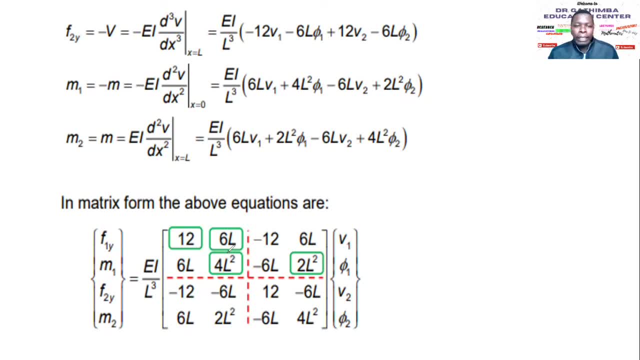 new video that's have come up. this work is not only for other graduate student and master student, but also for those people in practice who want to refresh, uh, what they've been learning. so, thank you very much. that's all for today, uh, and i appreciate for your patronage. let's continue. 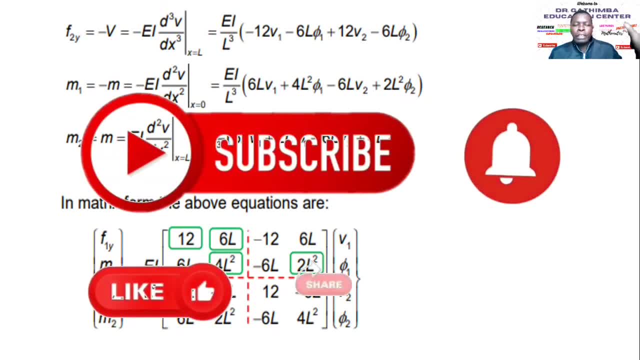 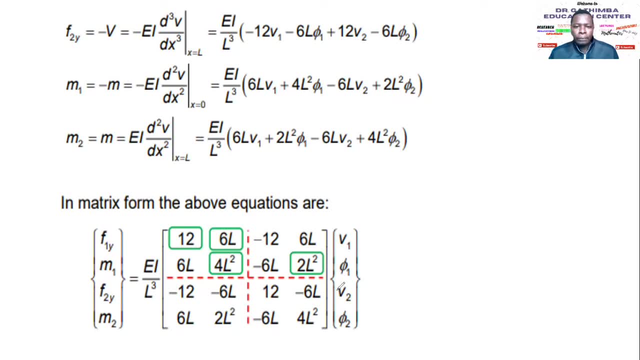 subscribing, sharing, share with your friend these videos, much it will share to facebook. here to share, to what up. let's spread the knowledge. thank you, god bless you until the next video. bye, bye, for now. 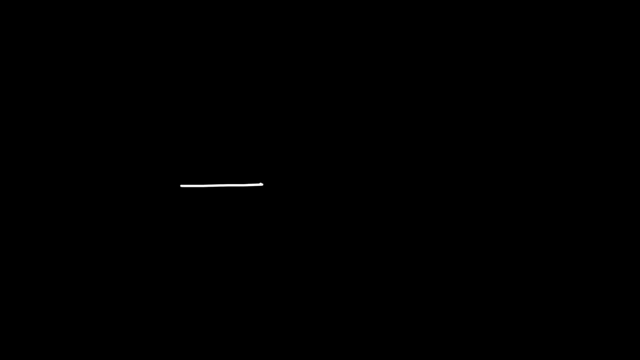 In this lesson we're going to talk about how to calculate the volume of a cube. So let's say the side length is 7.. What is the volume of this cube? Now we know that the volume of a rectangular prism is the length times the width times the height. 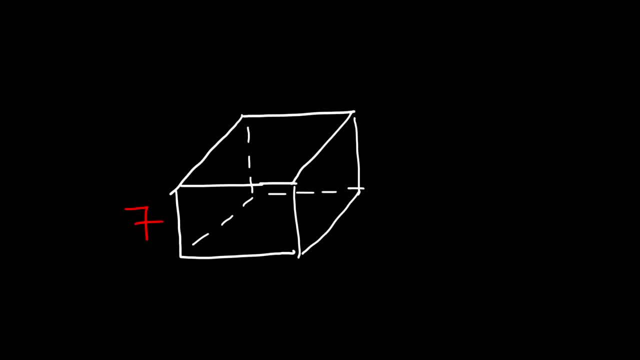 However, for a cube all sides are the same. So this is x, x and x. So it turns out that the volume of a cube is just x cubed. So in this example it's going to be 7 to the third power.